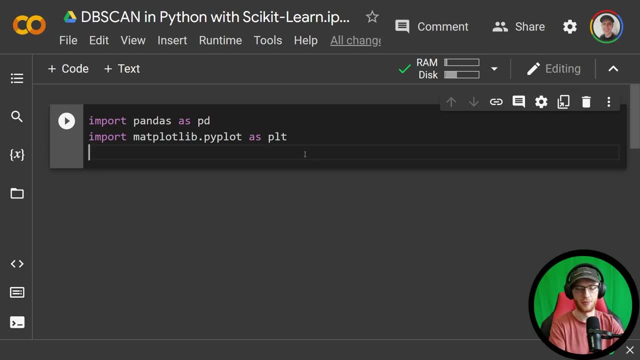 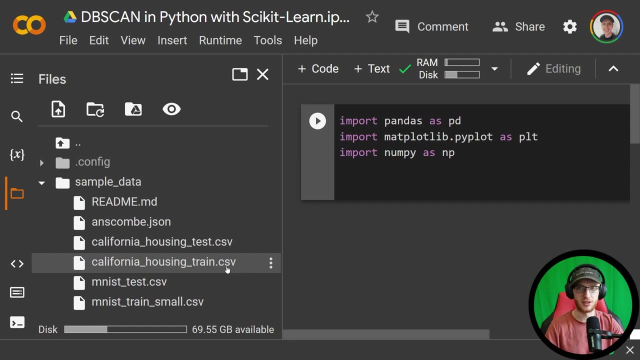 to be using plotly as well, although for now matplotlib is easier. Import numpy as np- And this is in Google Colab, by the way, if you guys didn't know. but you can use whatever site or IDE that you want, As long as you get this. Google Colab: California housing traincsv file. 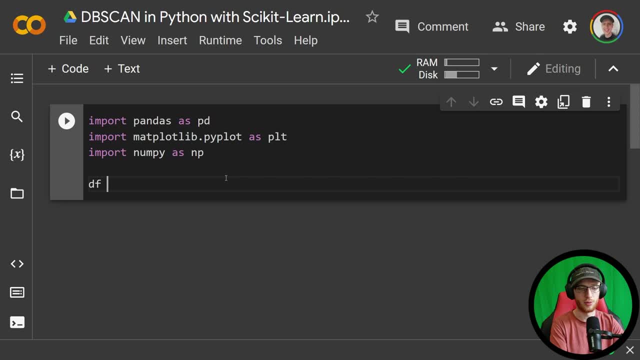 here I'm going to be using it. So we'll actually load that right away with df is equal to pdread csv, And then that file is located at sample underscore data slash: California housing traincsv. And then we'll just output The data frame df. Okay, so we just loaded that csv as a pandas data frame And basically what it. 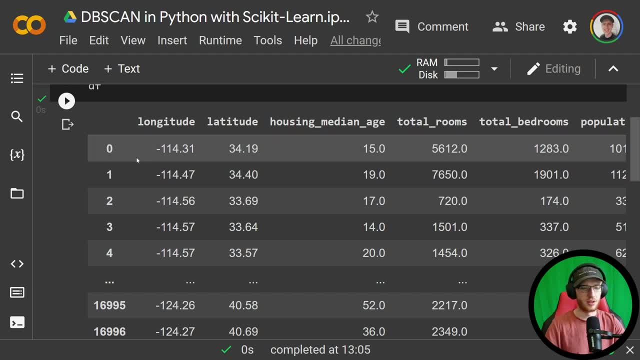 is. you've probably seen it before, But, as a quick overview, these are many different rows. in the data frame we have 17,000 rows And each of those rows has nine columns. Each of these rows represent a particular area in California which is marked geographically by its longitude and its 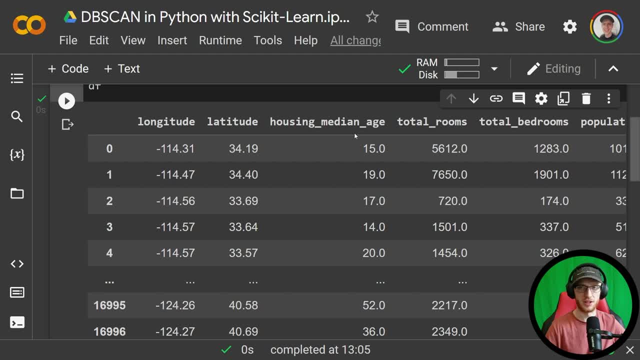 latitude And we have different descriptions of those areas in California, such as the median of all of the houses there, the total number of rooms in those houses, the total number of bedrooms, the population and so on. I'm not going to go over everything, especially because in this 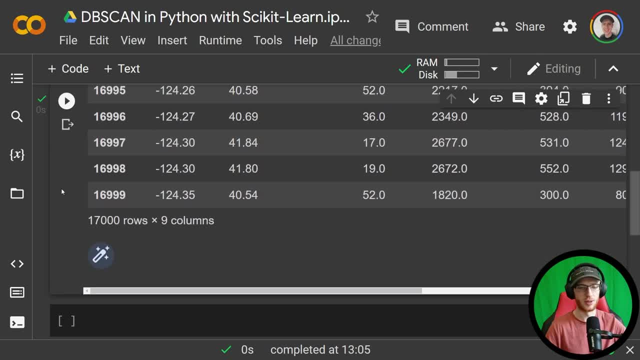 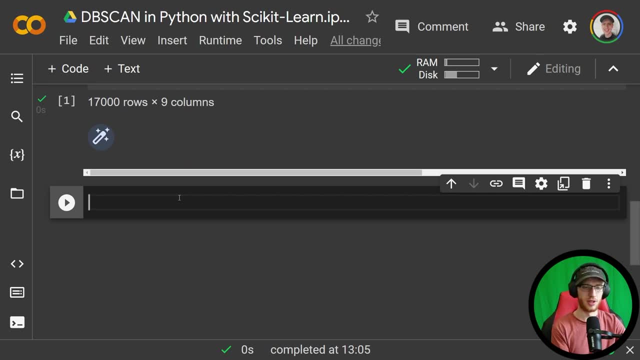 video. I'm not really going to use everything. we'll use a couple different pieces, starting with the latitude and longitude, Because a really nice way to graphically represent or show what clustering does is to use two dimensional graphing data, And this will be very clear in a moment. We'll get lat. 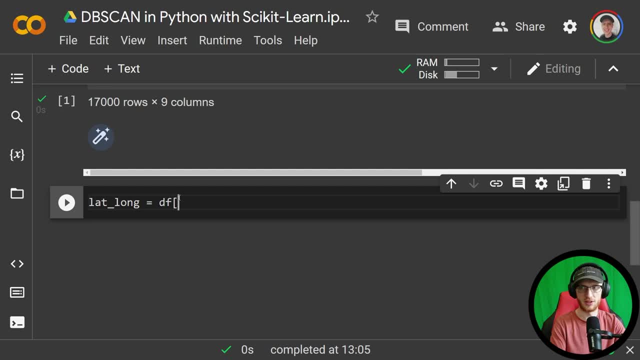 long as a subset of the data frame. And then we'll use the longitude and longitude as a subset of the data frame. With DF sub. we grab those columns- latitude and longitude, Okay, and we'll just for now separate that into two different variables. Latin long- we need to do long with two G's is 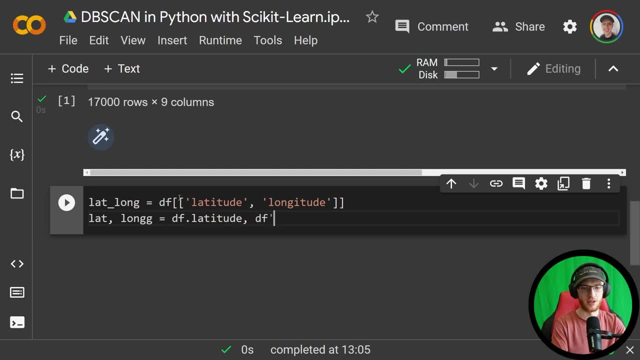 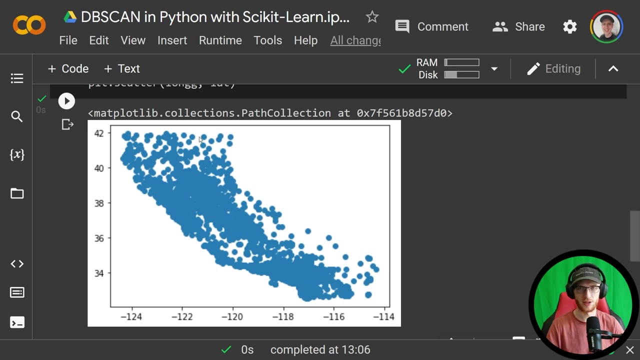 equal to DF dot latitude and DF dot longitude. Okay, so now that we have that, we'll just do a quick plot of PLT dot scatter with long and lat. it has to be in that order so that we get what California actually looks like, Since each of these points are an area in California with its 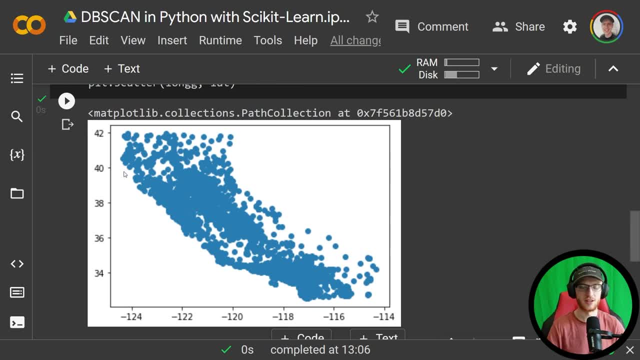 longitude on the x and its latitude on the y. this is actually going to show California, And so we don't have. if we fully painted in California, you would kind of fill in all the cracks and get the whole area. But these are just different areas in it. Okay, so why is this important? Well, we're 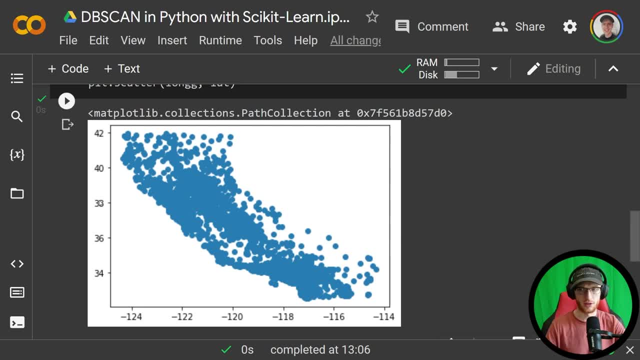 going to do a DB scan on these two, these two columns here on these two different variables, And so we can get loaded up with these two columns here, And so we can get loaded up with these two columns here, And so we can get loaded up with these two columns here, And so we can get loaded. 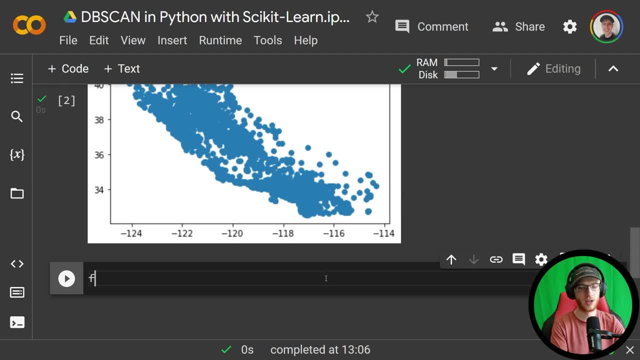 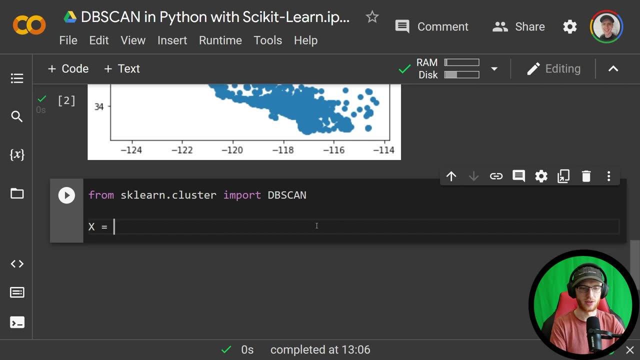 that right away. it's not overly difficult to fit a DB scan model. we do from SK learn dot cluster import DB scan. Okay, so that's their class for building and fitting DB scan algorithms, And we'll do x because, as always with machine learning, you usually have some matrix or 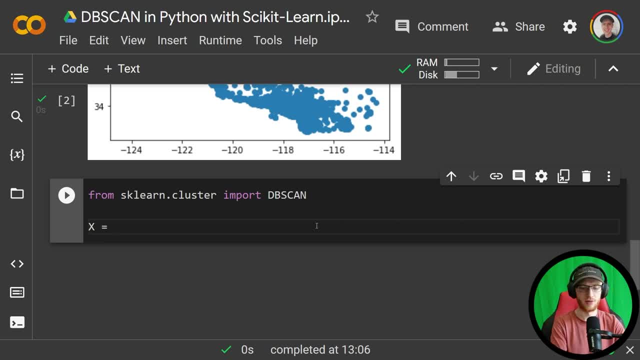 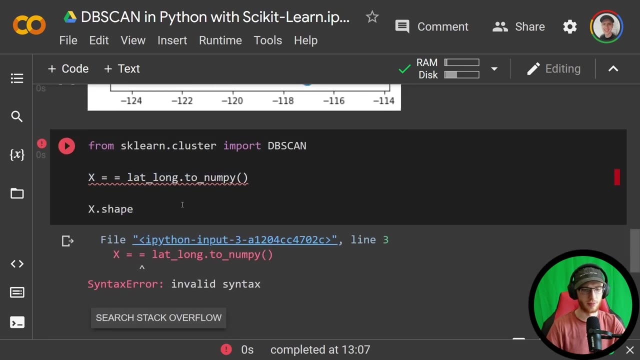 something that's kind of like a matrix, maybe a tensor we have for now. x is equal to lat long, which is that subset of the data frame dot to numpy. Okay, so That would mean that xshape better. be sorry, I must have missed something there. 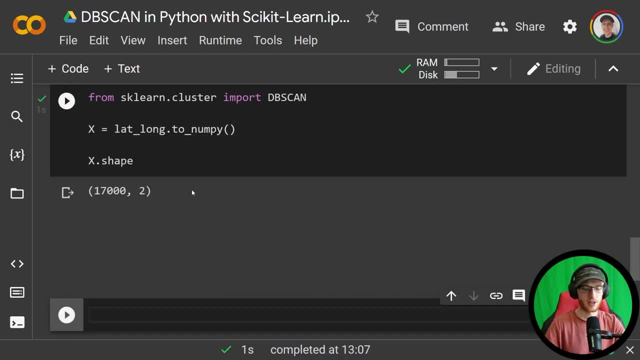 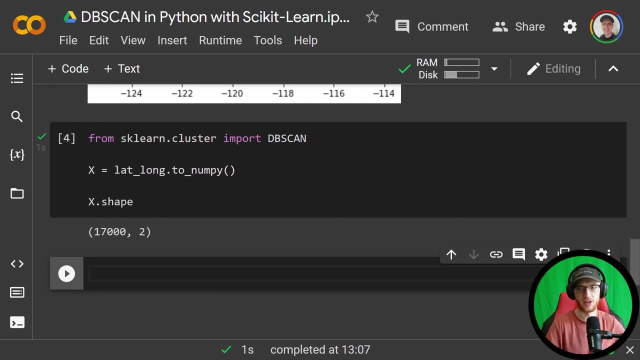 I just put two double equals or a double equals xshape here. it's going to be x is going to be a numpy array with that same number of rows- 17,000- and two columns, because it's just the latitude and the longitude. 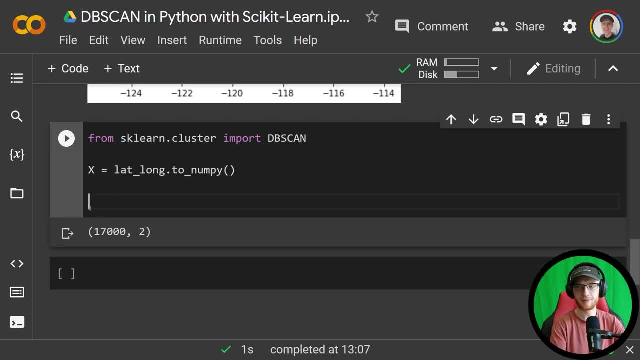 Now to fit the model which I'm actually just going to put in here. instead, we do grab it in a variable, We do dbscan, underscore, cluster, underscore, model is equal to dbscan. and then we set two different variables: We set epsilon and we set the minimum number of samples. 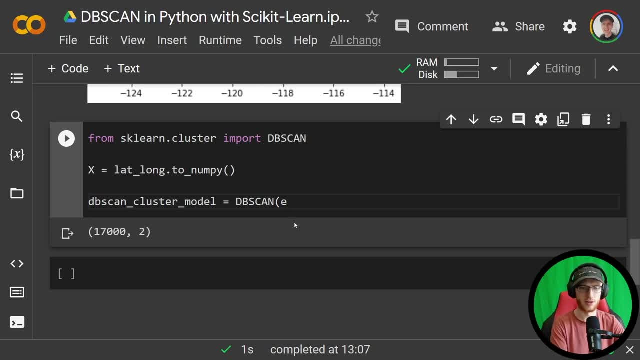 If you don't know what those are. well, you can kind of get along with this video if you don't really want to completely fully understand what they do. but I will give a little bit of a hint if you haven't seen how the algorithm works, in particular, 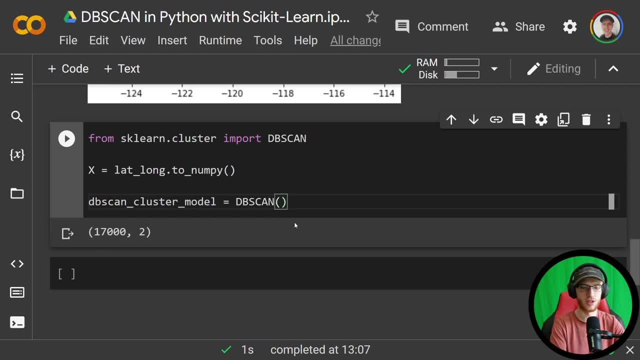 For now, I don't actually want to set anything, And so we'll just agree with their defaults, whatever they are. dbscan and we dot fit just x, and it's just x because this is an unsupervised learning algorithm. We're not trying to do some function that maps an input to an output. 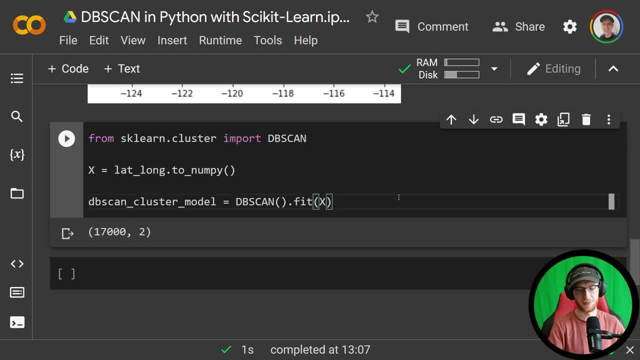 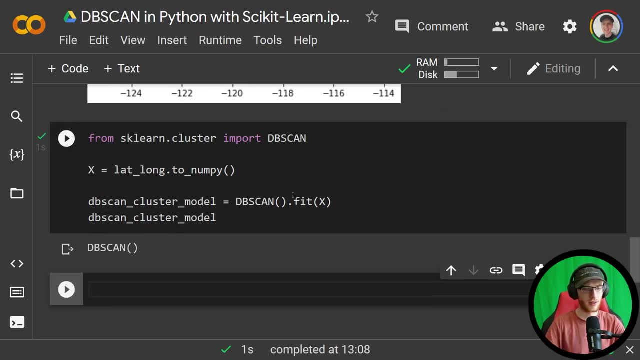 We are just doing learning something about the input space, So we dot fit x. Now if we output our dbscan cluster model, we will get just dbscan. Okay, it just fit a model and it didn't really say anything interesting, We fit. 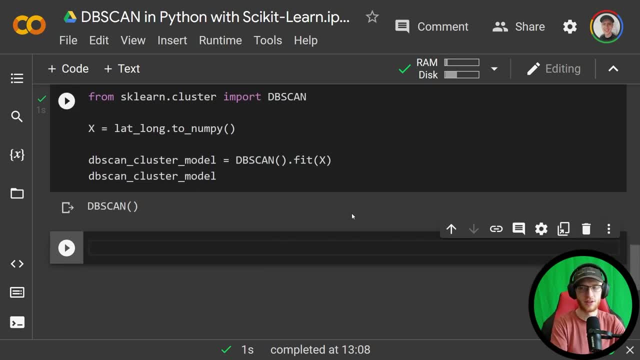 The model is interesting about this, but it doesn't tell us is that we have dbscan underscore, cluster underscore, model, dot labels, underscore. That's probably the most important thing for any clustering algorithm. The point is to label different things, label all of the points as a given cluster. 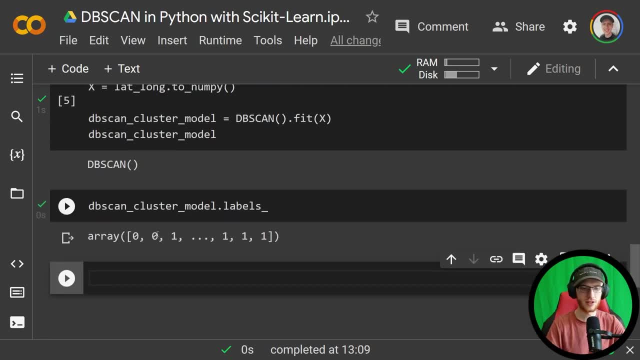 And so if we do, I'll just output that. for now It's an array, And if we convert this to a panda series, we'll actually add it to our data frame. If we do, df sub cluster Is equal to that labels. 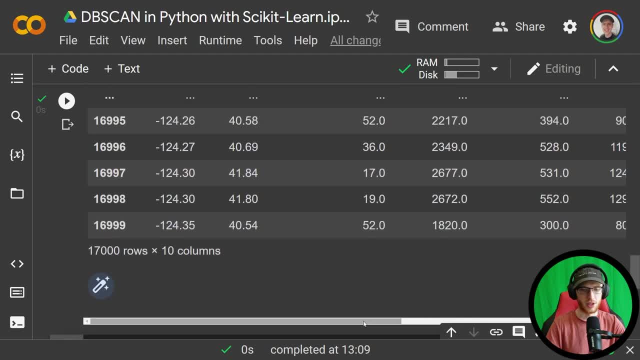 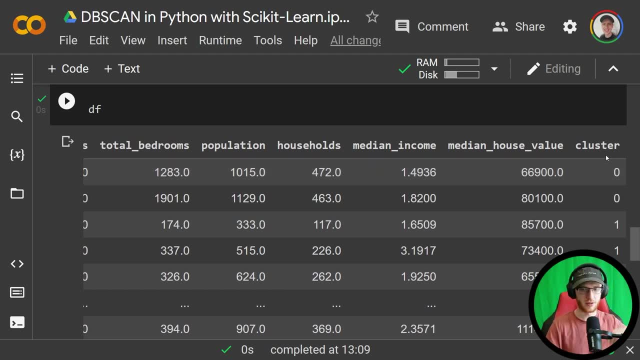 And then if we output the data frame, well, that shows that we basically put in a new column on the end there. That is each of our, each of our labels. And so I'm saying cluster because it's what cluster or what group it was assigned to what label it was given. 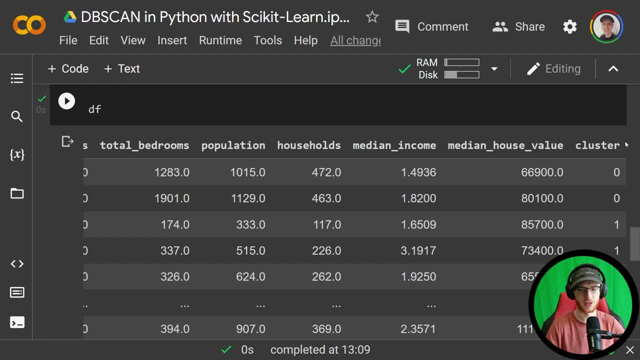 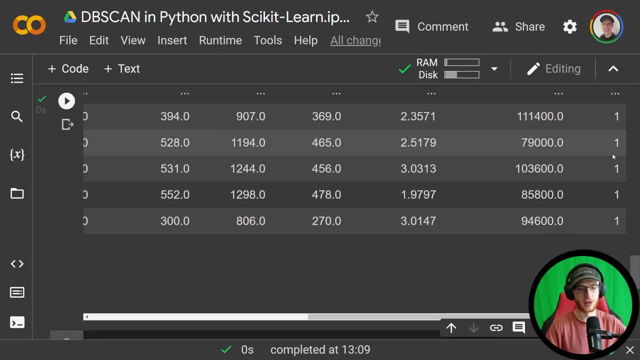 And it was assigned to each of the points. We have 17,000 of these clusters. We have one for every single point, And that's great, because what it allows us to do is what we've labeled: every single point, And now each of them belong to. 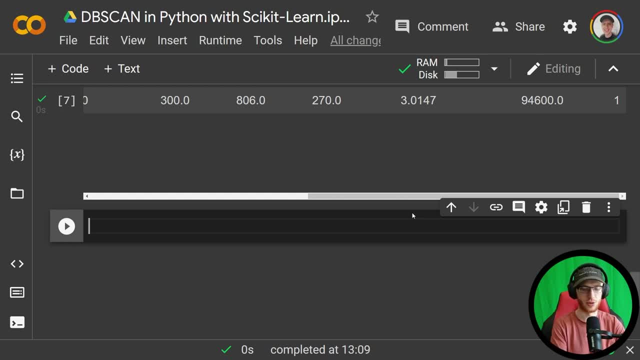 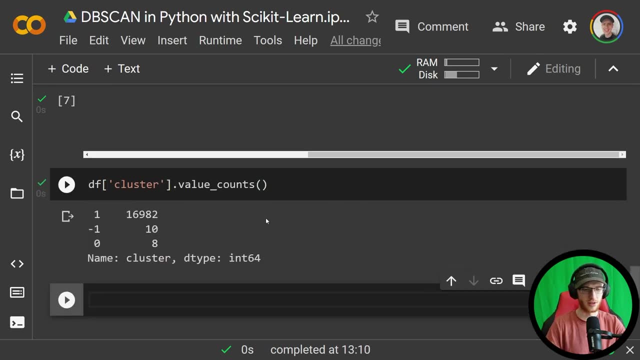 Some particular group. we can actually look at the different distribution with df sub cluster Dot value counts And what this does is this is saying that 16,982 of the points were assigned a cluster label of one, Eight were assigned a cluster label of zero and 10 were assigned a cluster value of negative one. 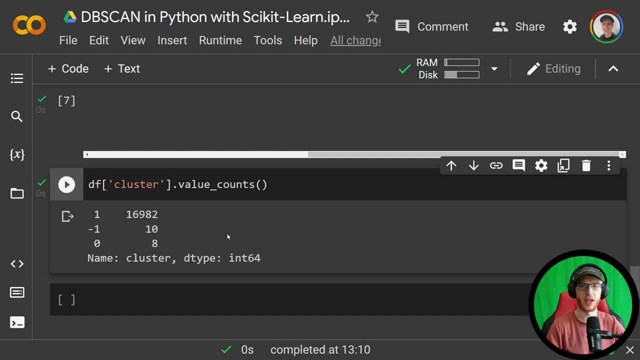 Basically what the negative one means is noise or, equivalently, outliers. It's basically saying: each of these 10. Points, they didn't really fit into any particular cluster. It's not like they're all part of the this, this negative one cluster. 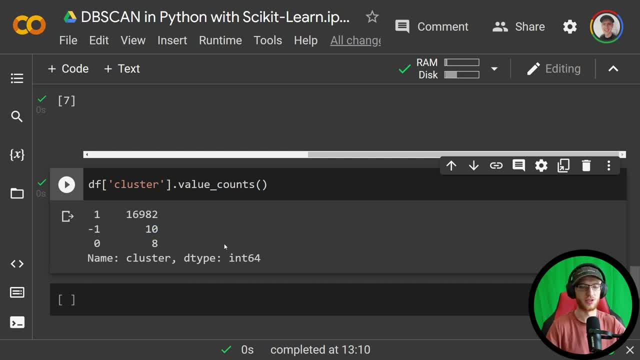 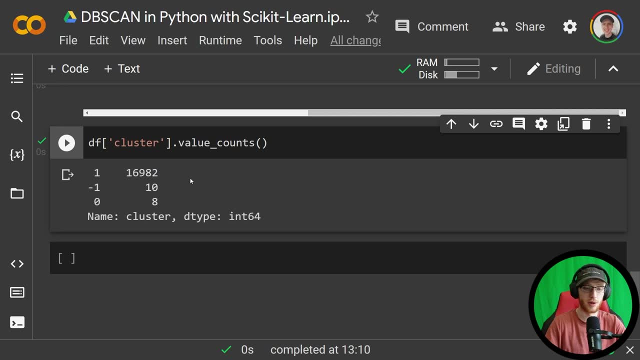 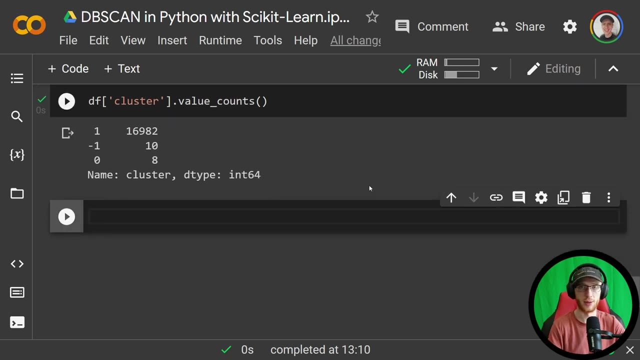 It's basically saying that they are all outliers, are all noise and we'll. we'll see that visually in a bit OK, but anything that's not the negative one. it's considered to have found a part of a particular cluster According to the parameters that we gave and the algorithm: DB scan with whatever epsilon and pin samples we gave. 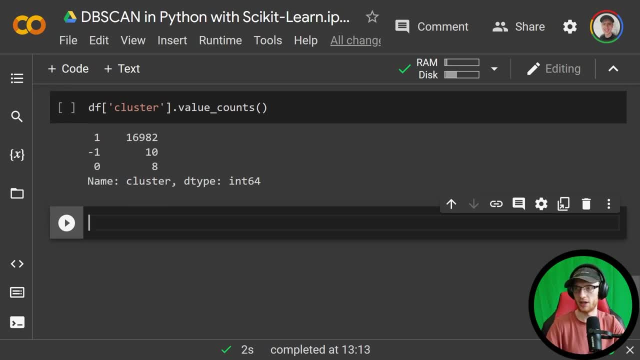 Again, if you don't know what those are, it doesn't really matter for now. So, basically, what we have Is the values of each of the different clusters, and these ones are noise and the other ones are part of some actual cluster. 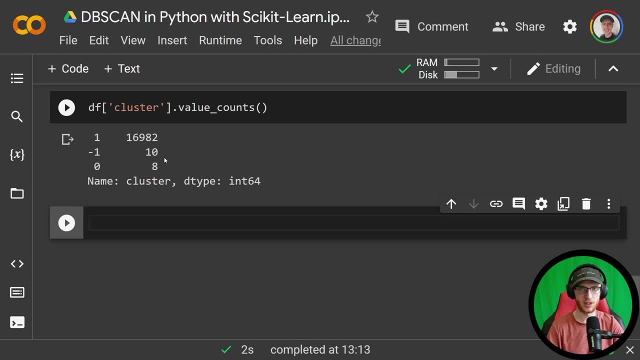 Well, what we can do is well graph, where we have the same plot as above and matplotlib. Actually, we're going to convert to plotly because it's a lot easier for this type of thing. But now we want to give each different cluster a color. 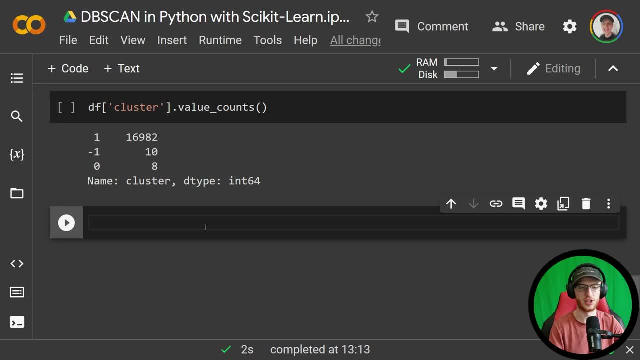 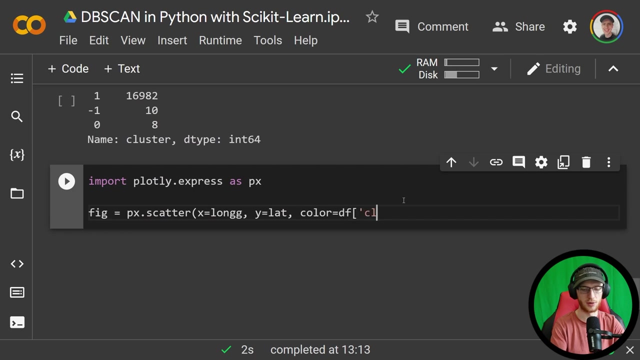 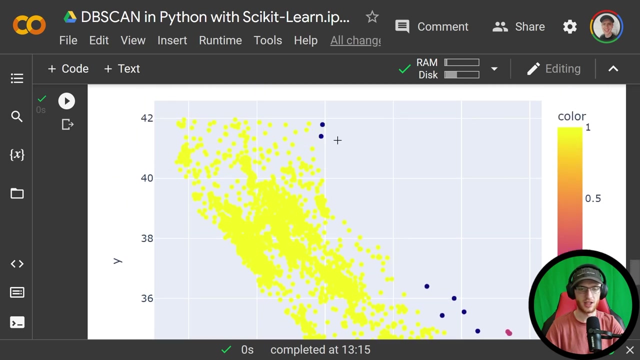 And plotly also does a really good job of you can hover over each point and see exactly what it is referring to. So we can just grab plotly with import, plotlyexpress As ps, Px, and we'll do. fig is equal to a px, dot scatter with x is equal to long, as before, y is equal to lat and, most importantly, here we set color equal to the df sub cluster and basically it's best explained by just showing you what this does. plotly is really smart about this color thing and since we set it like that, it's going to say that each of the, each of the values that have the same color, it is going to pick a color for them. 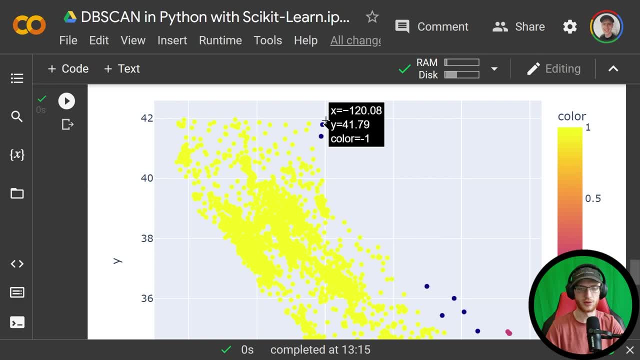 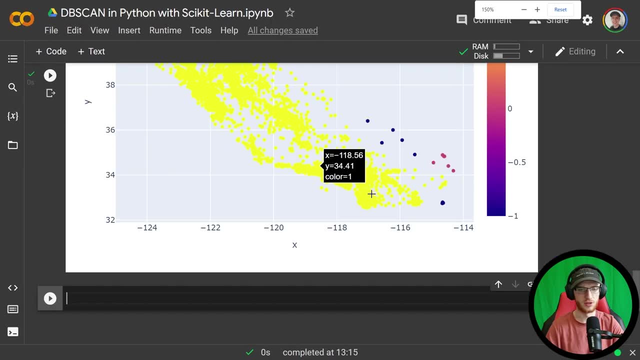 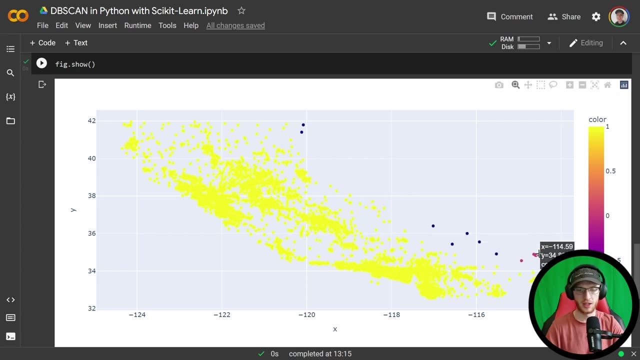 And so that'll be consistent. so each of these ones you can hover over and see that they're the blue ones here- are color of negative one. we can actually see that in this scale over here as well. I should really zoom out a little bit so you can see it better. but yeah, all of this yellow stuff, this is considered the one cluster and we had. apparently we had some tiny little cluster over here. now it turns out that this doesn't really make all that much sense and it's kind of up to you know, either a visual discretion or what we'll see later. 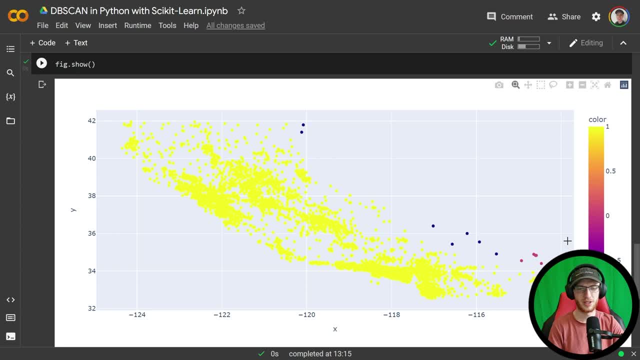 As some metrics as to what makes a good clustering model. but you know, this doesn't really make that much sense, like if I could get that. all of these are maybe a cluster because it's like inland stuff, and then we have some of the outskirts which are maybe outliers, but I really don't like that. it's just that there's this little kind of cluster over here, supposedly. and if this is your first clustering experience, then basically all we did is, according to some unsupervised learning algorithm, we colored each of the points or we assigned each of them to a group. 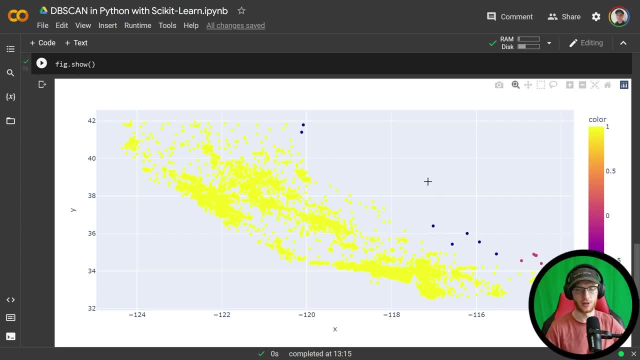 Depending on the DB scan algorithms parameters in this case, and it just it doesn't really make sense all of these different, the three different clusters that it has technically only two. we have these cluster: this cluster in yellow, this cluster in pink, and then these are outliers. what I would have preferred to see is, I don't know, just something different, and there is. if you go to scikit-learn's page, they have a really nice page on the different clustering algorithms and their effects. but I can tell you that 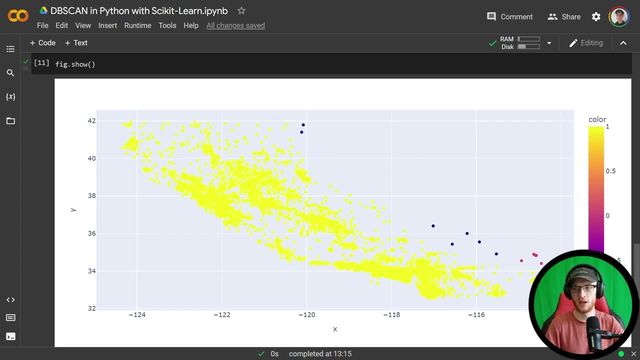 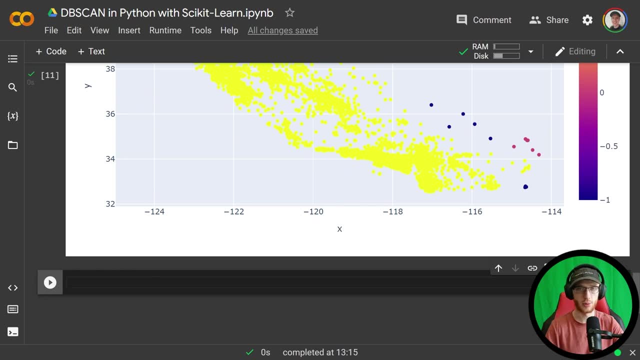 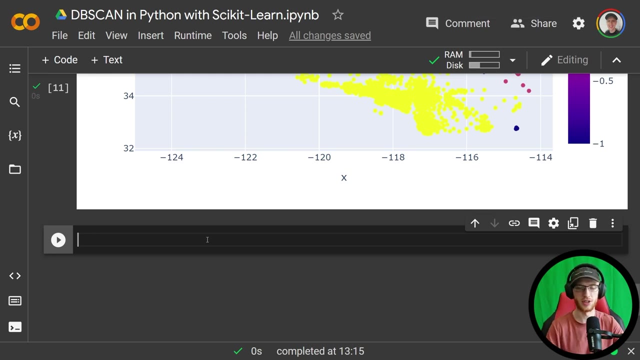 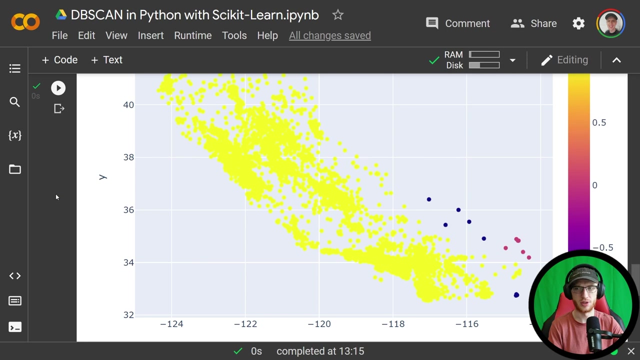 DB scan can do a better job of what we see here, and what I am going to show you in particular is that this is not going to get a good score on what we call the silhouette score in scikit-learn. okay, because we don't. because, in it, because this is an unsupervised learning approach, we don't have really any way of really easily verifying, like, how good this model is, at least one that makes really good sense. what I'm going to use, without explanation, is something called the silhouette score, which 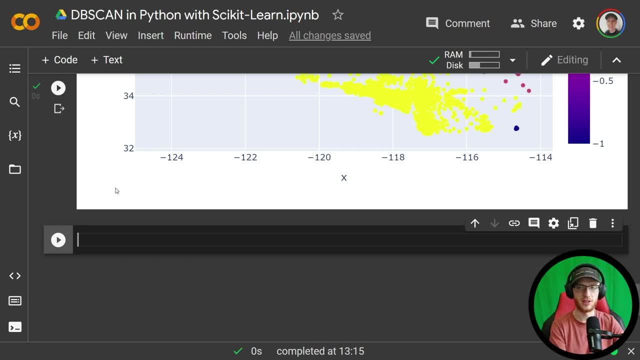 ELA, OK. So if we do from sk, learn dot metrics. we import still. so, huh, what silhouette score. and I'm just going to write it as SS, because that's really irritating to write over and over again. and if we do SS, If we 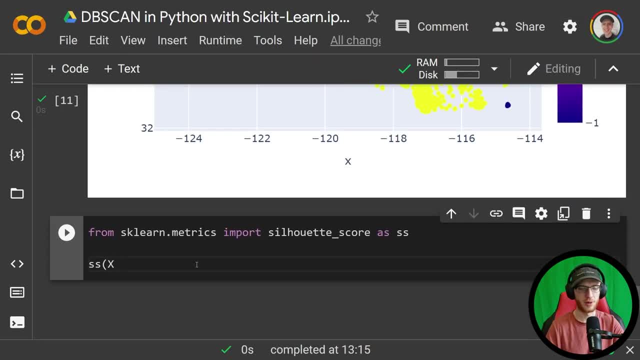 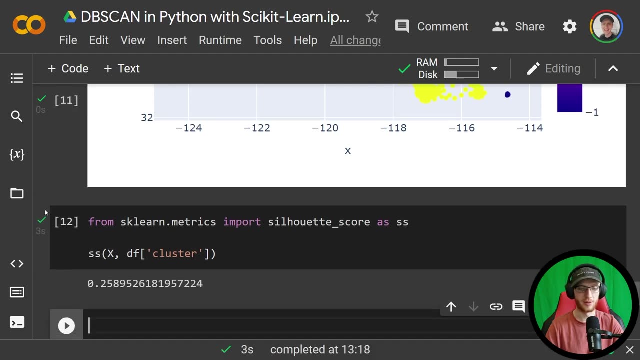 we pass it. i should probably zoom in a little bit more again. we pass it. our input matrix x and the cluster labels that were outputted, df sub cluster. that's a different way of getting those labels that we got. it's going to output a score for us and it actually takes a little bit of time to. 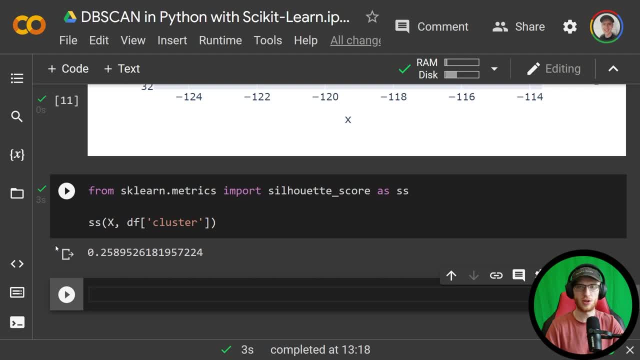 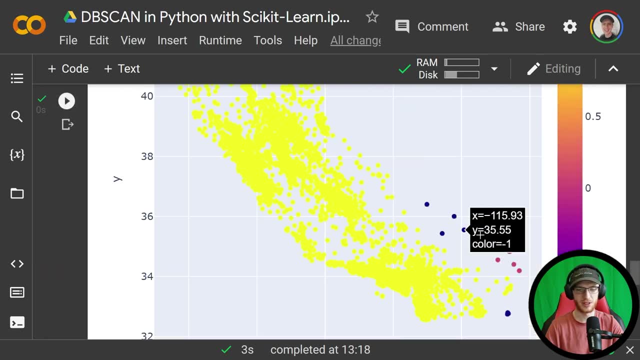 compute that it gets 0.26, which is okay, but you could definitely get better for this, this cluster model like this. it makes a little bit of sense, but it's not amazing. so what do we do? how do we try and how do we try and adjust this? well, db scan: you can play with two different components. 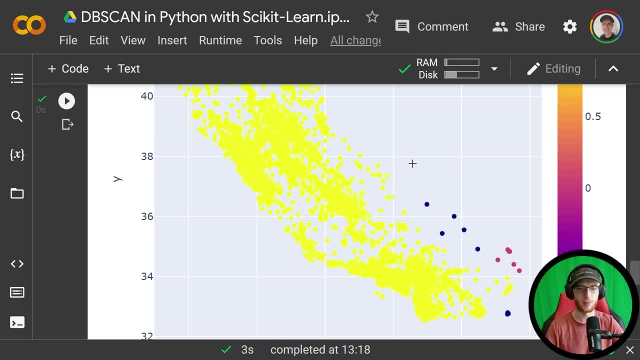 you can play with epsilon, which is the distance that marks a core point, and you can. you can play with min samples, which says how many points, how many points are required for something to be a core point. epsilon also does slightly more than that, but it's a little bit more than that. but it's a little bit more than that, but it's a little bit more. 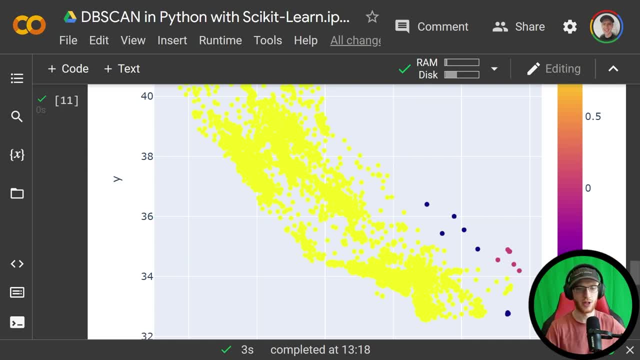 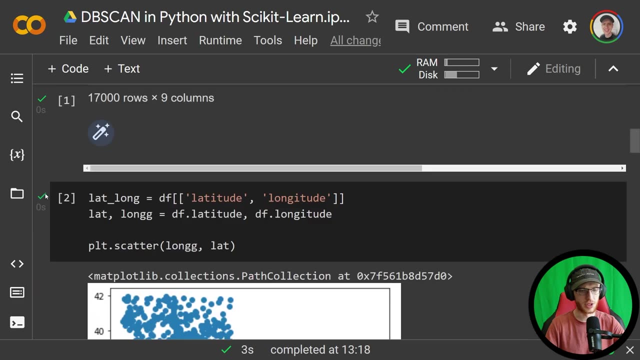 not really a big deal. as i said, i don't want to explain the full algorithm here. you can check it out in in my, my other video, and that will explain, okay. so, most importantly, we do need to play around with epsilon and min samples and we could do this randomly. for now we could go back to where we. 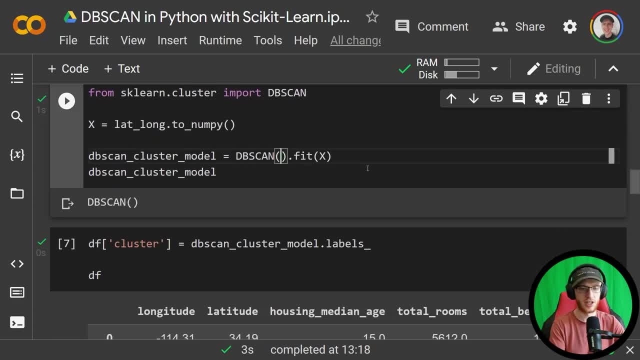 change that. sorry, it's a little too far. uh, we didn't change anything here at all and their defaults, whatever they are. we're going to change epsilon and min samples. so if we do epsilon, maybe we'll set it equal to a smaller 0.2 and we could also set, um, maybe min samples to be- i don't know- 15, and when that's, let's run. 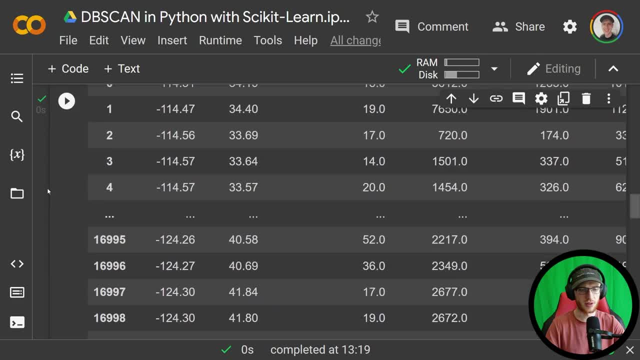 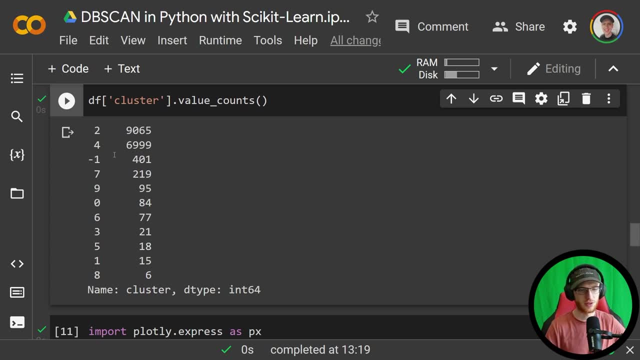 that again. okay, it's not going to look all that different for now. what we should see is a different number of clusters, okay. so here's all the different distributions we have. there's a 84 get assigned to the zero label, 15 get assigned to the one, 9065 to the two, and lots of different ones. what's? 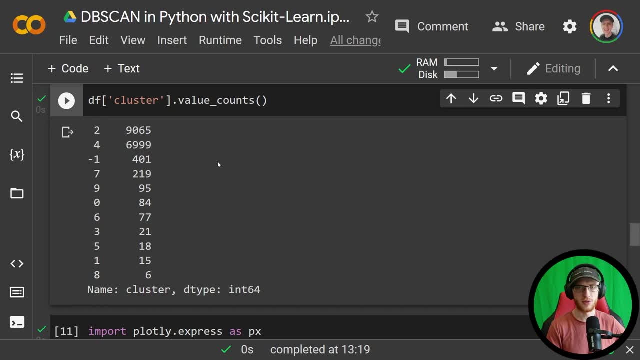 important for db scan, as you see here, is that we have a lot of different clusters and we have a lot of different clusters and we have a lot of different clusters and we have a lot of different clusters here is that we don't choose beforehand the number of clusters that are going to be outputted. 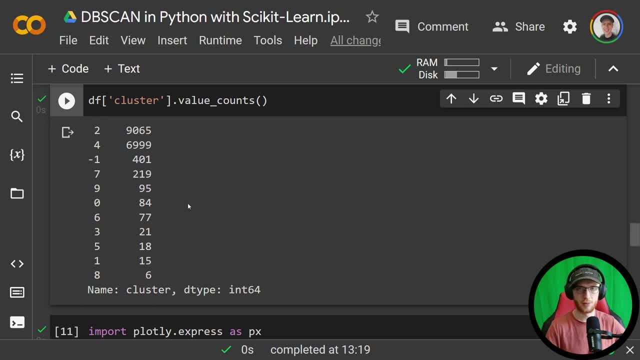 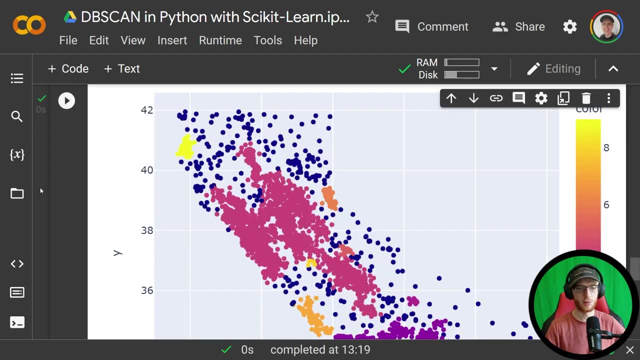 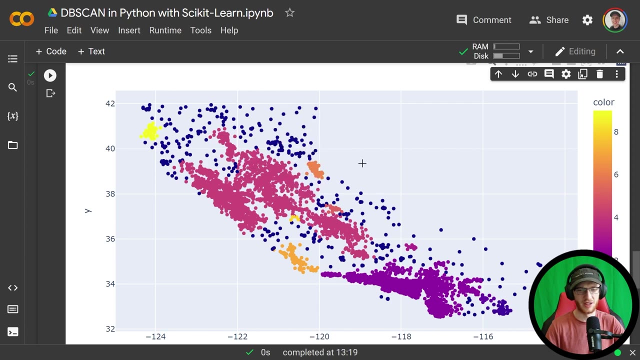 and so that is kind of figured out automatically by the algorithm, depending on those parameters that you gave. so it got a lot more clusters and we can run this again, and what we see now is something that, oh, makes a lot less sense than it did before. i really don't like this at all. um, yeah, this, this doesn't make a. 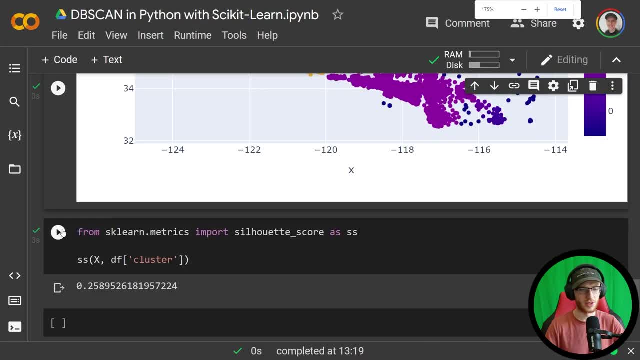 lot of sense for california. and so what do we get? according to a silhouette score, well, marking our visual guess, it is about the same. i guess, according to this metric it's still not very good and i guess it thinks that it's okay. but i i tell you i really don't. 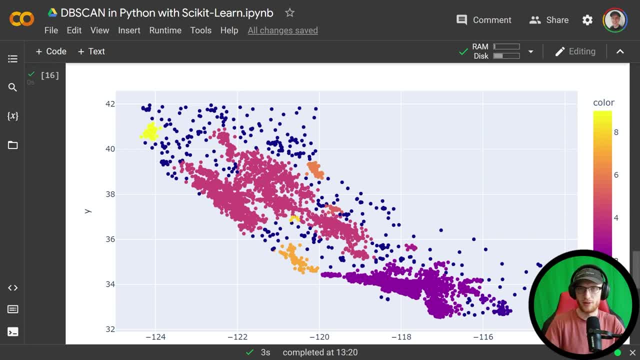 like this result. now, although we may not get a perfect result for any data set, and i'm not trying to pretend that this is something that you can really get a super awesome result on for california- what is important is that we can optimize this somehow, and to do that well, we 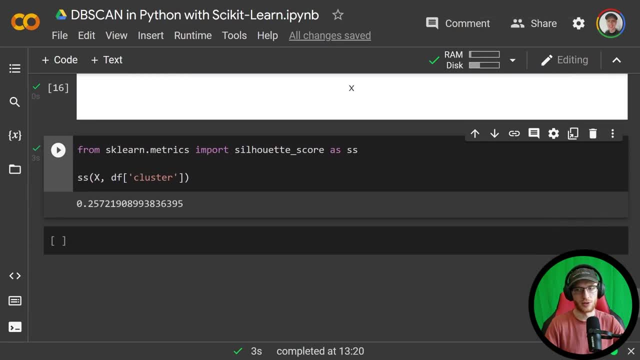 usually use in machine learning the formula that is the first one, that's a scan of data set, and we in machine learning some sort of a grid search and you may see some other techniques for finding epsilon and min samples in db scan, but what's easiest in to code, even though actually what's 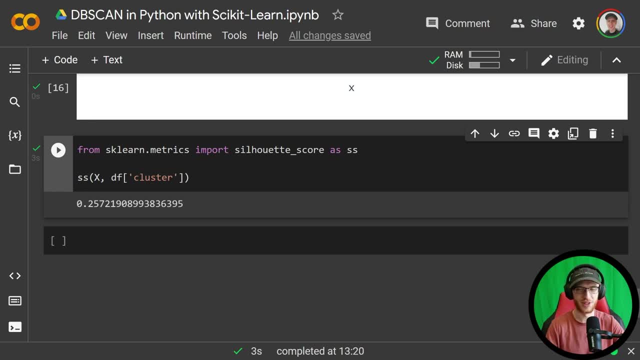 coming up coding. it's going to be a little bit confusing, i i apologize for that, but it is really really useful, so just stick with me on it. we're going to optimize via a grid search on epsilon and min samples and if you don't know what a grid search is, it's not very complicated. 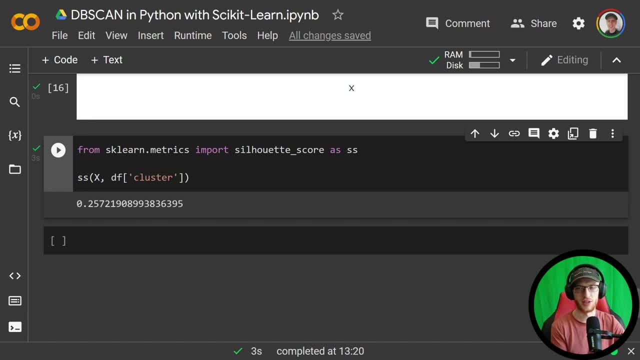 it basically just says: try all possible combinations of these two lists of things. and so if we get, say, a bunch of epsilons to try, epsilons is equal to nplin space- with we'll say starting at 0.01, you don't want to start at zero because you don't want zero distance. that would. 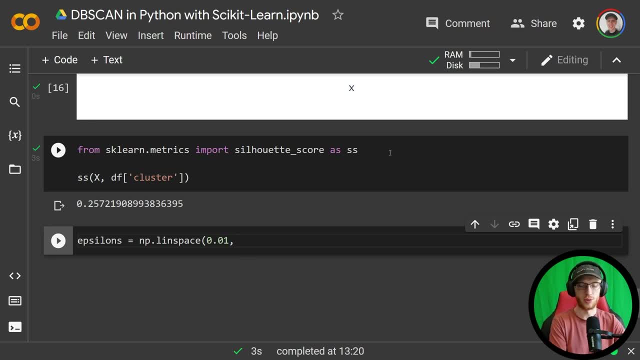 not make the algorithm happy. nplin space 0.001 and we'll go to one and then we'll do num number of those is equal to 15.. so that our various epsilons to try: are these different values here? okay, so spaced evenly. 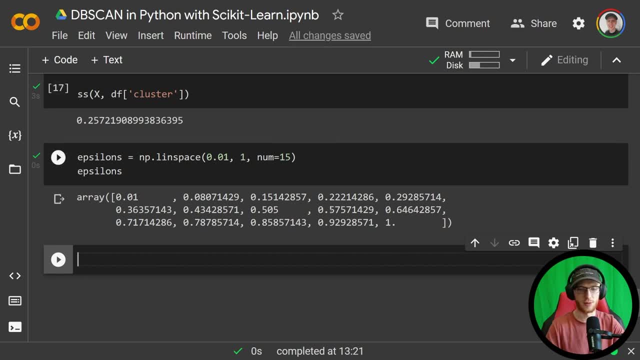 between 0.01 and 1. we have these different epsilons to try. we could, of course, get more or less, but i don't want this to take super duper long and i do want to get a decent search as well. we can get. 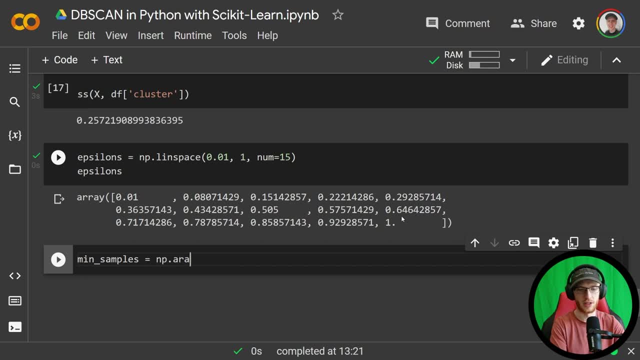 different min samples is equal to npa range between 2 and 20 and a step equal to 3. this is just something i played around a little bit on my own and you can feel free to check it out. if you play with them by yourself, there's really no limit to how many different values you need. 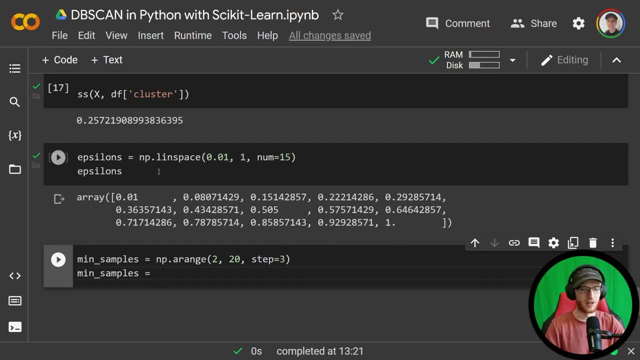 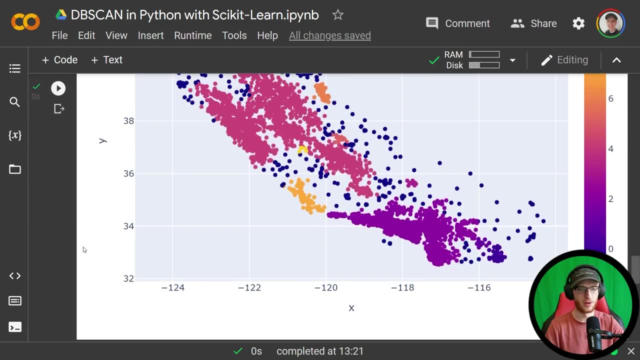 i'd pick more than one, so at least two, and generally between zero and one for epsilons. we'll actually get to that because this isn't standardized, although longitude and latitude are pretty much on the same scale, so we don't have to worry that to that about that at the moment. 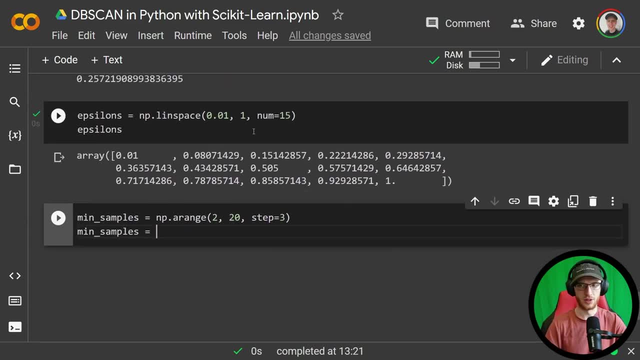 we will in a bit, but still, either way between zero and one is going to be probably proper, and min samples so some values between, say, 2 and 20.. are decent to try. so and i don't need an equals min samples, we're just going to do 2, 5, 8, 11, 14 and 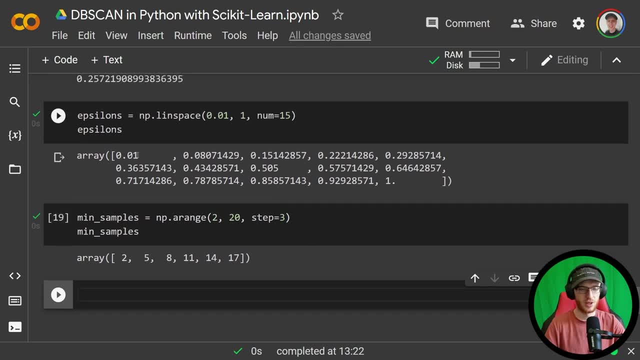 17, and so a grid search is just going to try, well, 0.01 and 2, and 0.01 and 5, and 0.01 and 8, and all of those combinations, and then 0.08 with 2, 0.08 with 5, so it's just trying all these different. 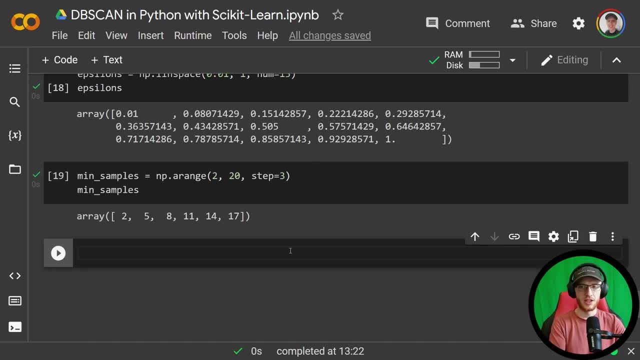 combinations to try and get a good one. and an easy way to get those combinations is just import and mean so you convert the envelope to one and you can do combinations. combinations is equal to the list of iter tools, dot product um with epsilons and min samples. 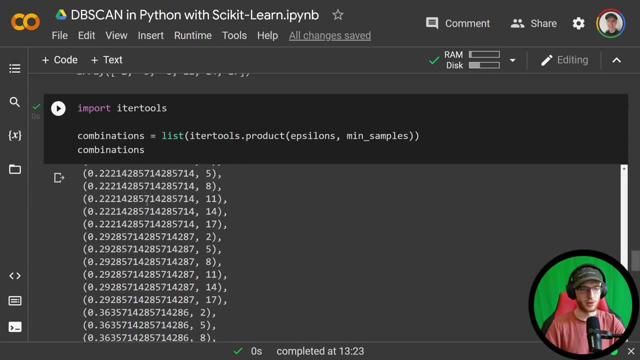 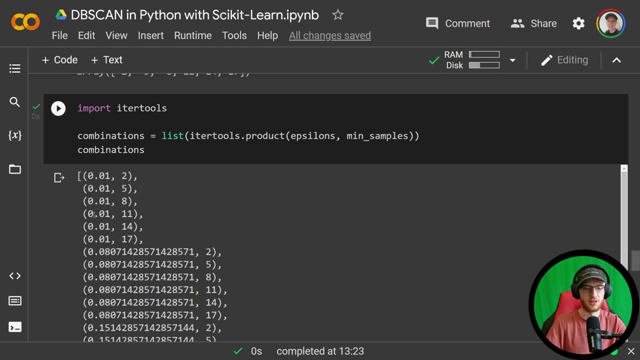 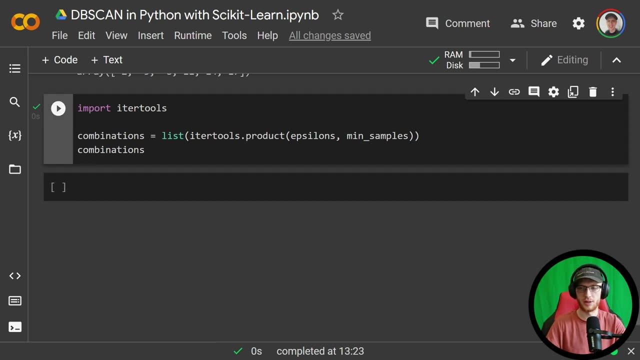 okay, and then combinations. combinations is probably what you'd expect. it's actually with tuples, and so it's a list of the tuples, of all those combinations, as i said. so in the first column you have all of your different Epsilon's, different min samples and the combinations between those. Okay, I'm going to exit that. 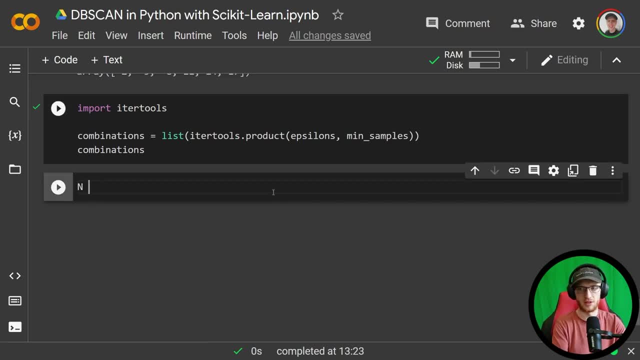 because it is kind of a long list And just so that we have this we're going to do: n is equal to the length of the combinations And we can see that n is equal to 90 in this case. Now, this is by far the most complicated coding we're going to do, So stick with me. But most tutorials won't do. 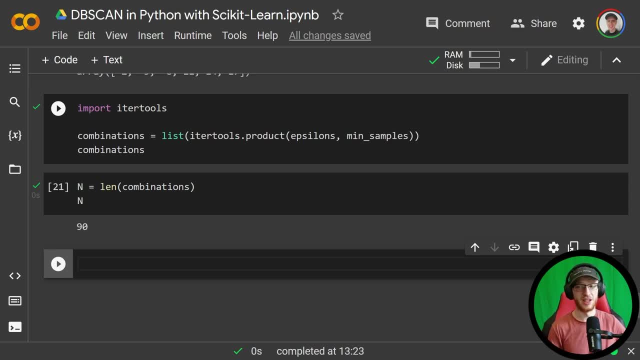 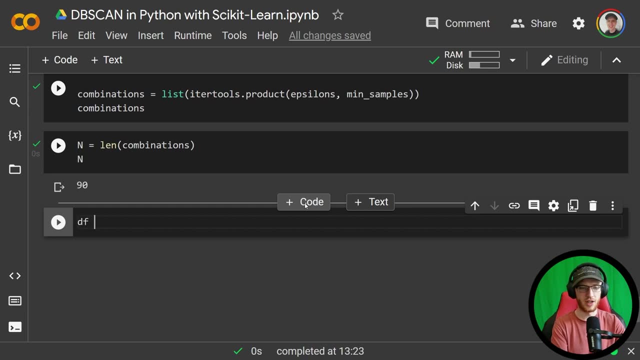 this because they don't place an importance on finding an actually good model and showing you how to do this. I will show you how to get an actually good model for db scan So we can do, define, get scores and labels If you, if you get confused in this, just wait it out And I'll. 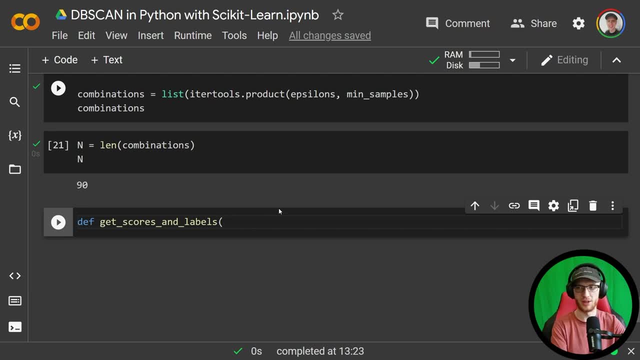 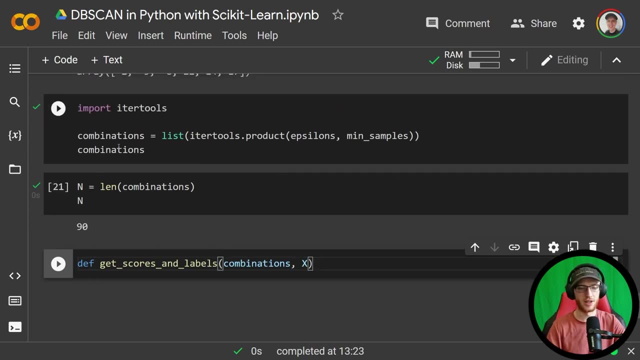 explain everything I promise, Define, get scores and labels with combinations and x. Okay, so that. combinations you- you can probably guess what Pat will be passing in this- combinations over here And x. that's kind of the same or possibly a different matrix. 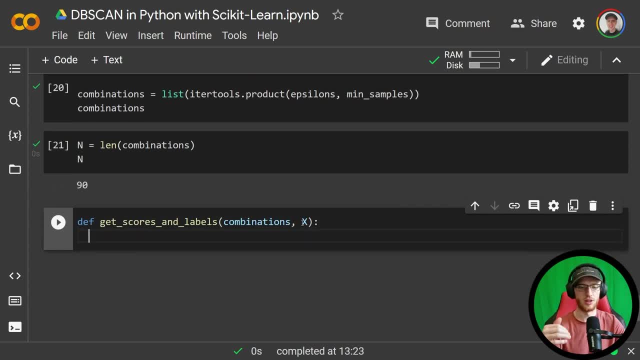 As before, it should be a numpy array which represents a matrix as an input. So we'll start with these two empty lists. lists scores is equal to empty list and all labels list is equal to an empty list. This is going to be a list of scores. that is going to be for each db scan model. 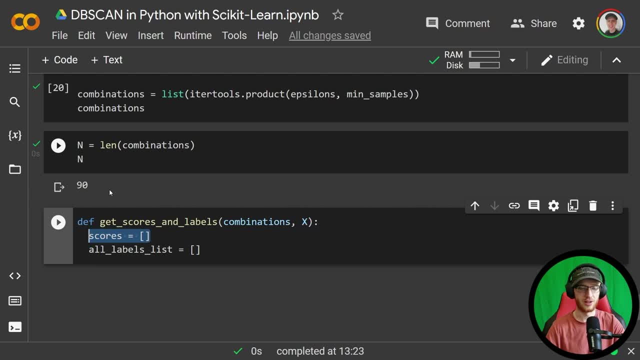 that we try. So we're going to have 90 of those because we'll be trying 90 combinations And this is going to store all the different lists of labels. So the first component of this will be the labels associated with the first combination And the 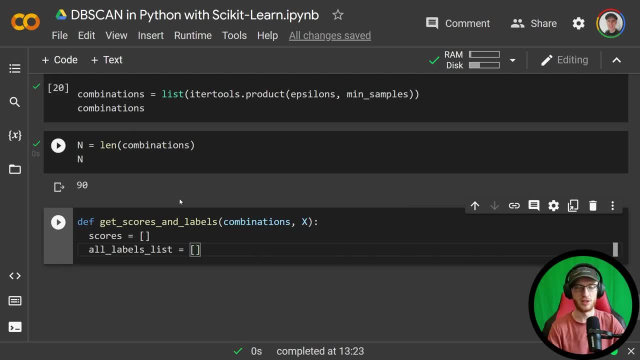 second, the labels associated with the second combination would be the second element. we're just going to try many different combinations of db scan, Or we're just going to try many different db scan models with each of those combinations and record its main results. Now what we're going to. 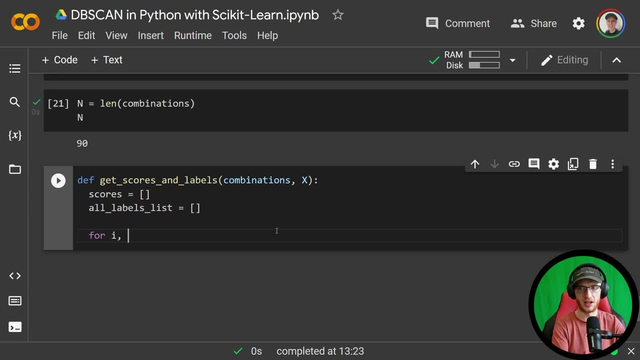 do is first a for loop where for getting I and epsilon and num samples In enumerate the combinations- okay, if you haven't seen enumerate before. basically it's just the best of both worlds for iterating through something. This is a list of tuples And so we get the index starting at zero and then going up until the. 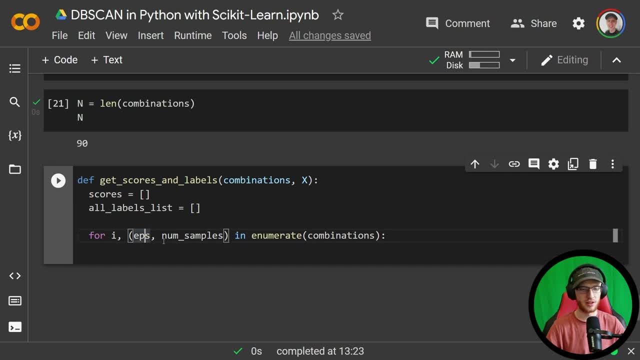 length of it minus one, as usual, And this we get immediately access to epsilon and num samples, which is that particular combination that we're going to be iterating through. since we're enumerating through the combinations Now, we'll make a model db scan underscore. 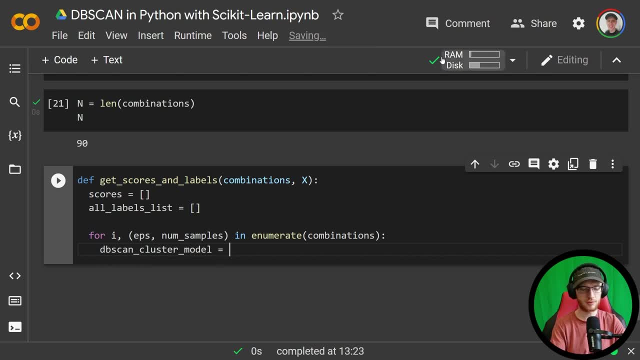 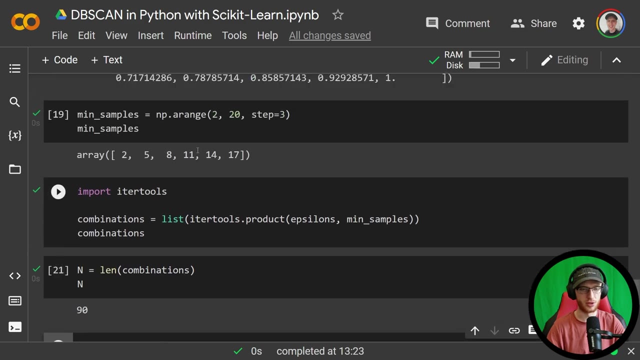 cluster underscore model is equal to db scan And then epsilon is going to be equal, equal to epsilon, whatever epsilon we're iterating through, or whichever one from the combination we have which is dependent on. you know our combinations and we're doing a. 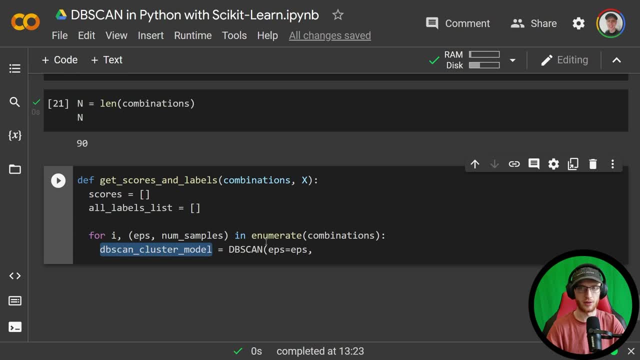 grid search. So we're going to be: each time we get a model, we're going to be storing its results And we're going to be trying to find the best one. So min samples: it's going to be that: min samples. 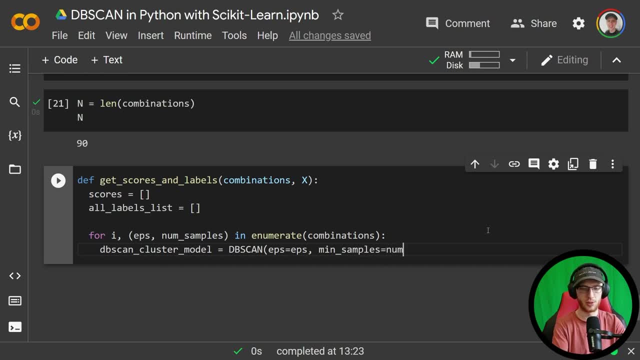 that we're doing number by number with our set label that we have, that we're entering through as well, which will be num samples. then we'll dot fit with x, just like it is above. look at the labels. which is equal to the DBScan db scan cluster model. 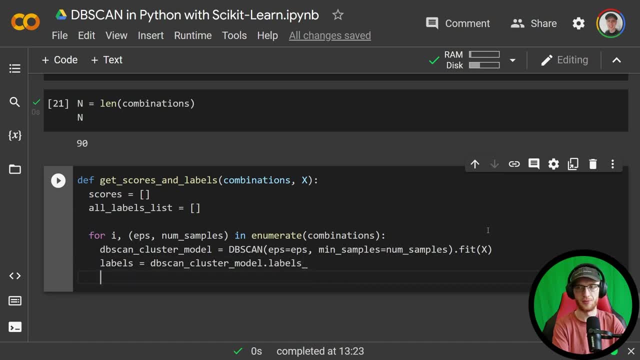 dot labels underscore, just like it was before. we'll convert that to a set labels underscore. set is equal to the set of the labels. And then what we want to do to count the number of clusters whole, First it's going just: number of clusters is equal to the, uh, the length of the label set, except then to get the. 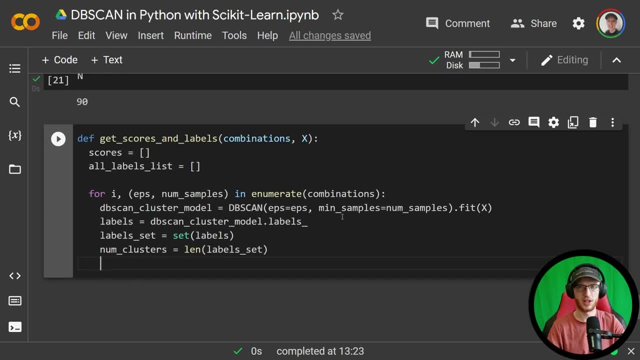 actual number of real clusters, because if something's assigned to negative one, then it's not really a cluster, it's just noise. the number of real clusters is going to be reduced by one if the if negative one is in that set. so if negative one is in the labels set, if we actually 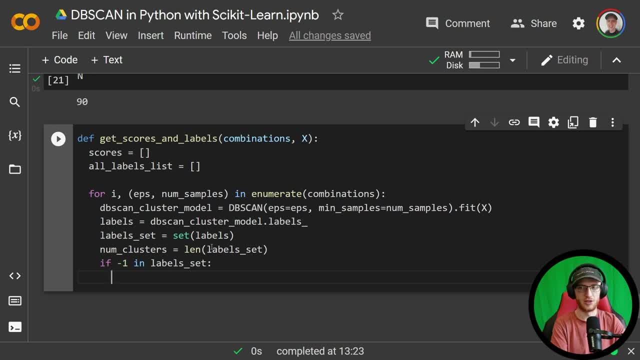 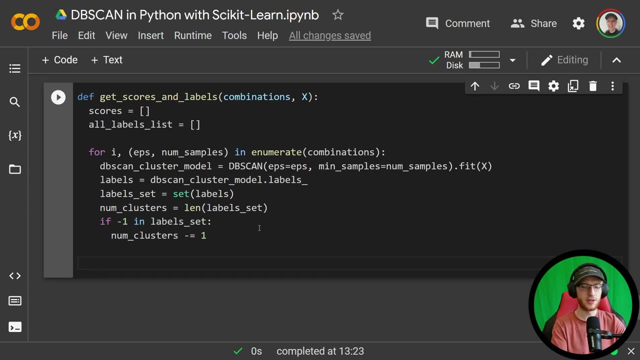 labeled anything as as noise, then we're just going to decrease num clusters by one. minus equals one, okay, so why do we need that? well, it's because we don't really want to make or even spend time on models that make really no sense, and it's a little bit up to us as to what makes no sense. 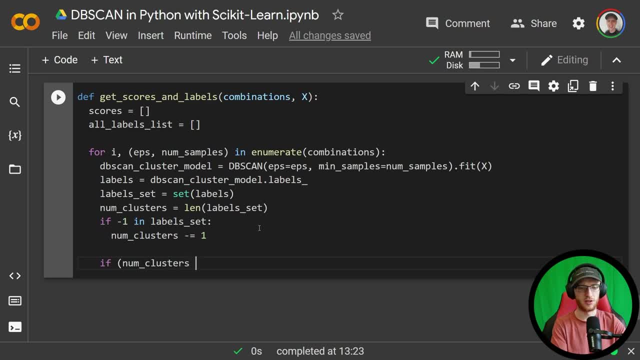 but i don't want to do. if num clusters is less than two, so if we, this is even disregarding the noise already. so this basically means if we've only made actually one of the models that make really no sense, then we're just going to decrease num clusters. 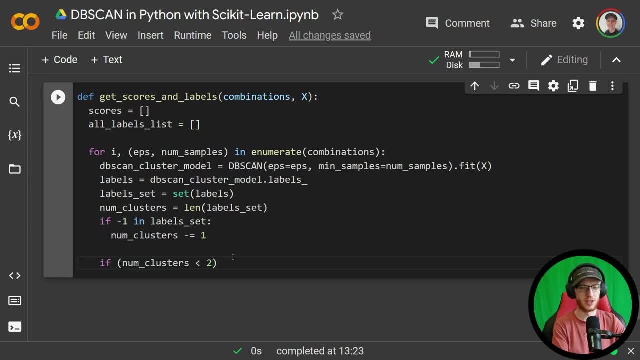 one real cluster. i don't like that model so i'm not even going to consider it um. if this is true or something, that's a little bit up to our discretion. technically, there should really no be, not be an upper bound on um on a number of clusters. it's not really realistic to say: 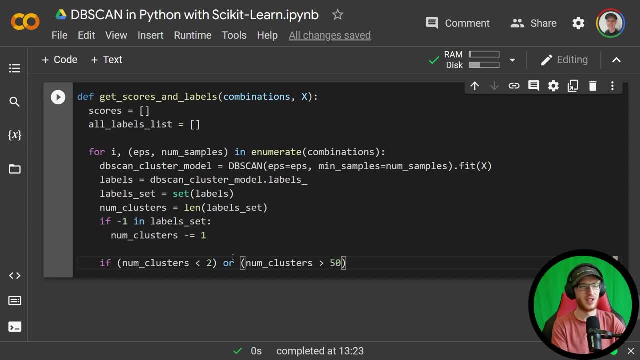 hey, if there's something bigger than, say, like 50 clusters or so, this is getting a little bit complex. now again, many people would disagree about this practice. it's not. this is not some set in stone practice. uh, but it's not a set in stone practice. it's not a set in stone practice. 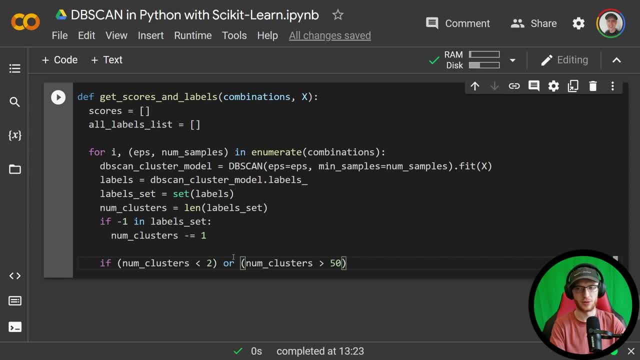 but if something, if we're getting something massive for this particular problem, i'm just going to ignore it. now, what we're going to do is: if this is true, then what we want to do is ignore it, to ignore this properly. we will still append some garbage into the scores, because we're still 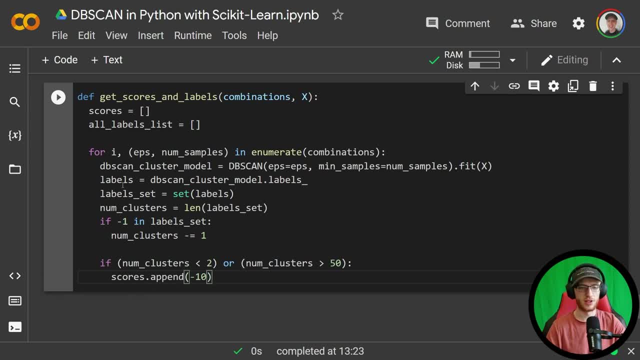 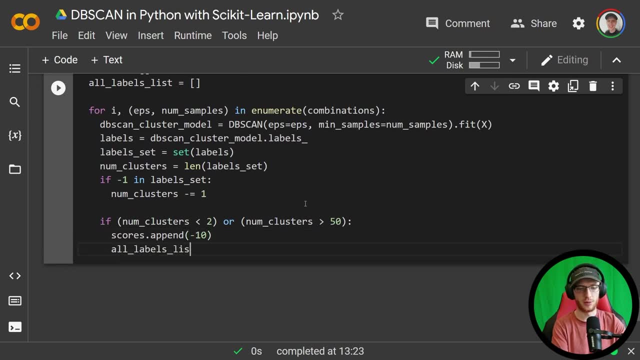 trying to calculate this is. this should be the score for this model, but we're going to ignore it. so we're going to add some noise here and we'll also match this up with all labels. list, dot, append- uh bad, so we're going to append again just some garbage into this list, which basically just says ignore. 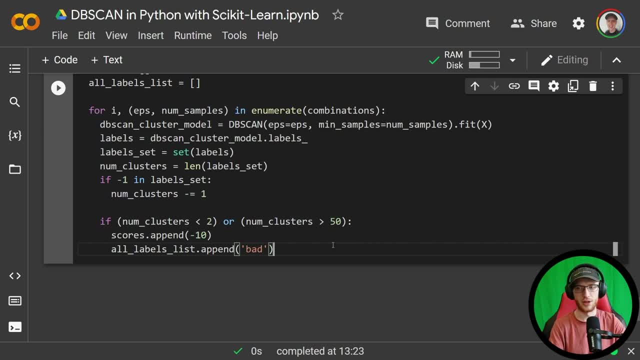 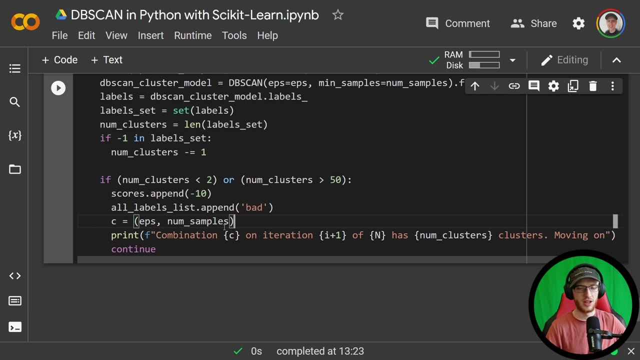 this score, ignore this set of labels because we're not using this model. if we wanted to, we could make this nice printout, which i'm actually just going to copy in because it's not super relevant. if we do, c is equal to that tuples. there we can output this nice string which basically says: hey, i want. 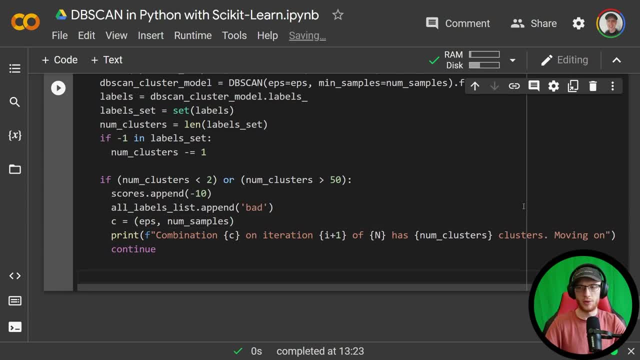 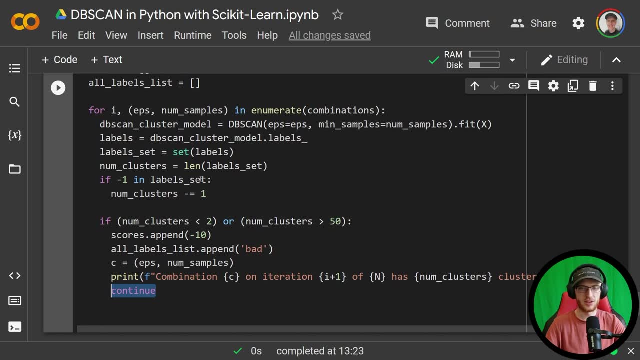 to still just write some output to see what we're doing. okay, so now what we want to do is basically- since in here we have a continue when we initialize our behavior, so we handle our output, which basically just says: if something's wrong here, we're just going to go over to the next iteration. grab the next epsilon and number. 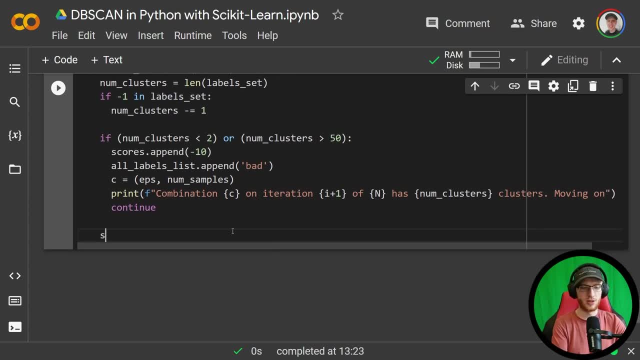 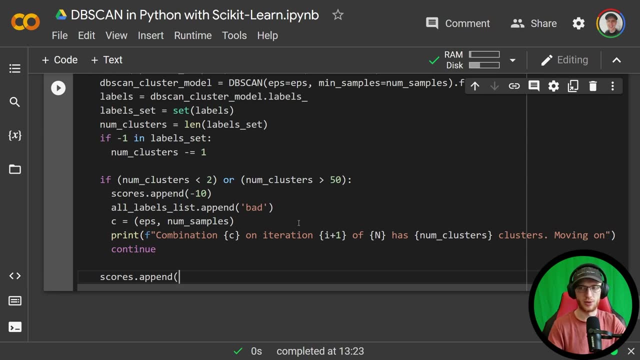 of samples. well, if we here down here, we actually do care about the model, and so that means we should have some score since we already made the model up here. so well, scores dot. append the actual score that we got, which is computing that ss with x and the labels. that's how we did it. 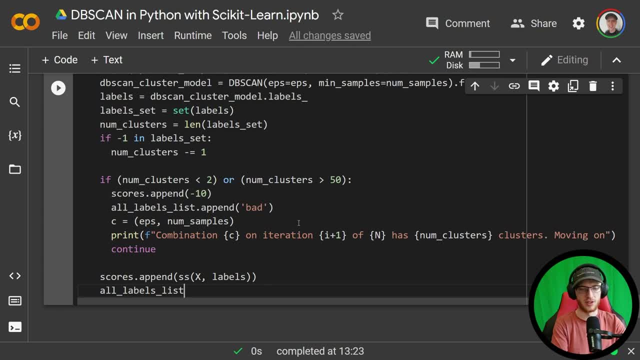 all labels list. all labels list dot. append with the labels. Okay, so now here we added the score for that set of parameters And we added the labels. Now we're going to add a nice print here as well. I am actually going to copy this in here as well, because it's not super important, But 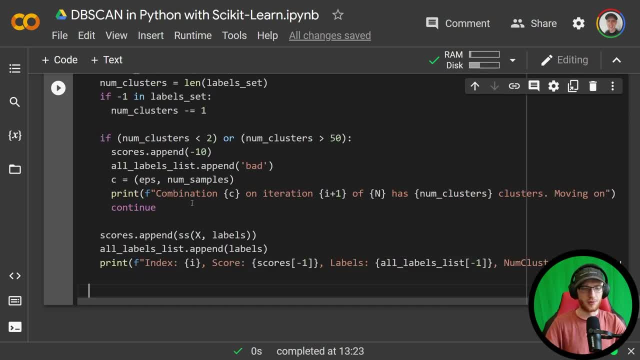 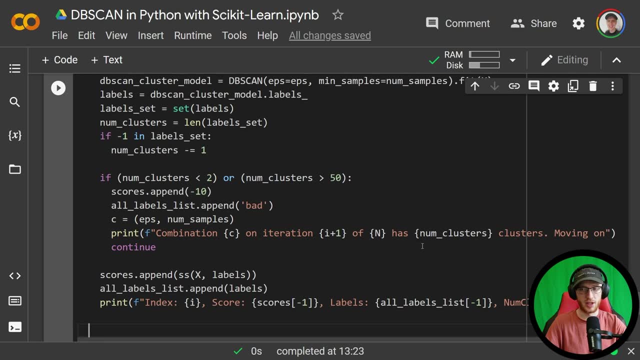 again. I'm just going to really skip over that. Okay, so now we want to do is return things that we actually care about. What do we care about? Well, we probably care about the parameters that were best, the labels that were best and the score that was best. Okay, so what parameters? 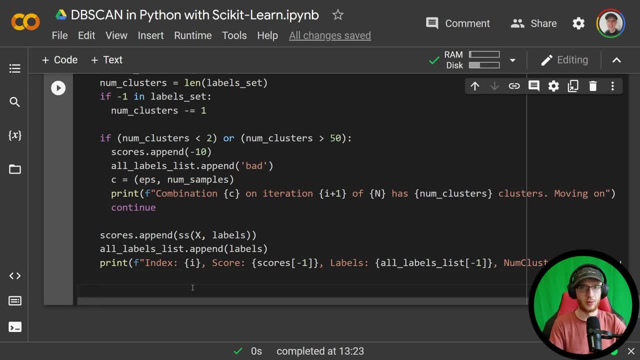 got the best score and and what labels were associated with that model. The reason we need to actually get the labels right now. instead of running the model again, we could technically just extract the same parameter, the best parameters, and then run that model once more to get the best. 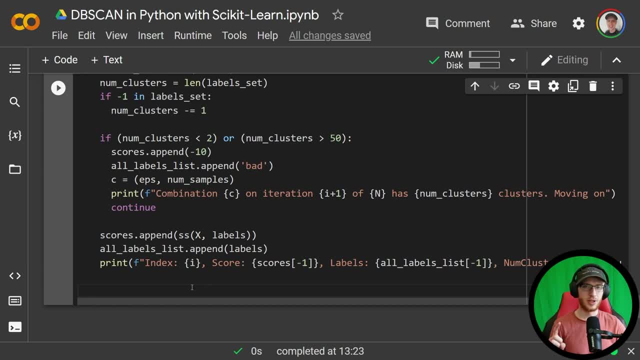 one. Well, the reason we need to actually get the labels right now instead of running the model, the reason we want to actually extract the labels, is because db scan is not deterministic due to the way it sequentially makes something kind of at random, a cluster. Well, that's going. 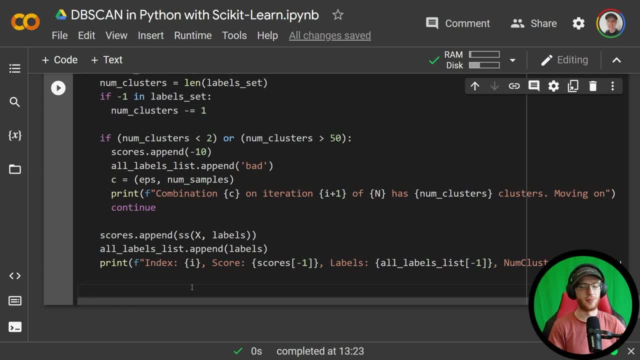 to make it not necessarily get the same output every time, And so we want to get the labels that were associated with it the first time that it ran. So what do we need? to make sure it's best? Well, we'll do best. index is equal to the numpy dot arg max of the scores, because that says: 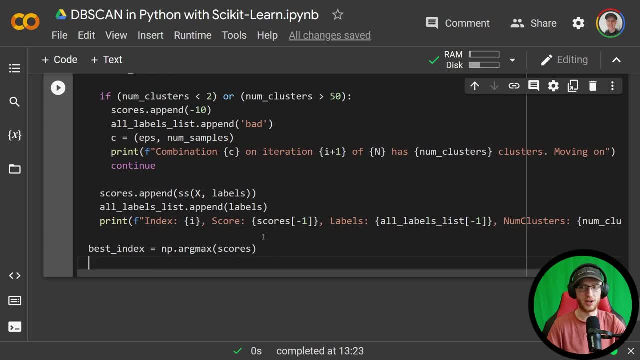 which index maximizes the scores. that's the one we care about Now. we can basically just index everything. with this we'll do best parameters or our epsilon best, best combination. basically, best parameters is equal to combinations, So the best index, because that's the combination. 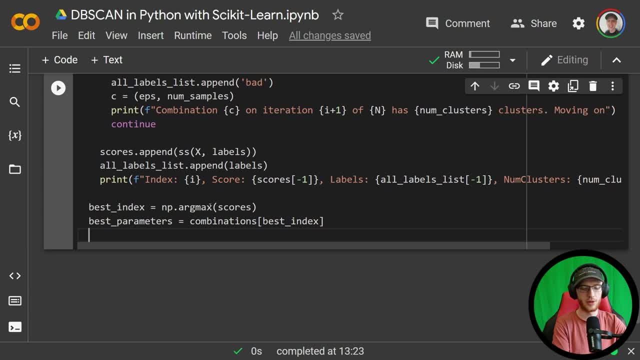 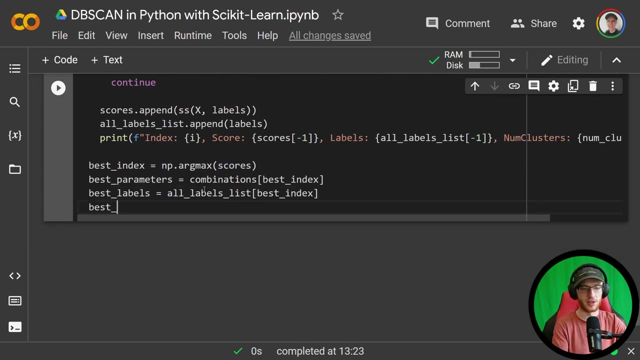 that has the best score. Now we can do: best labels is equal to all, all labels list and then give that best index again. so those are the best labels that are associated and finally we'll also get the best score, which is just going to be scores sub best index. okay, very long function, i know. 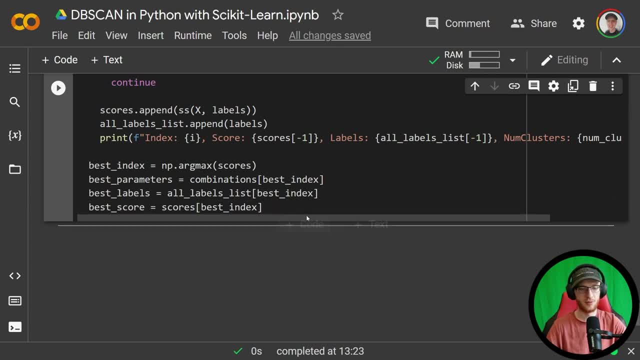 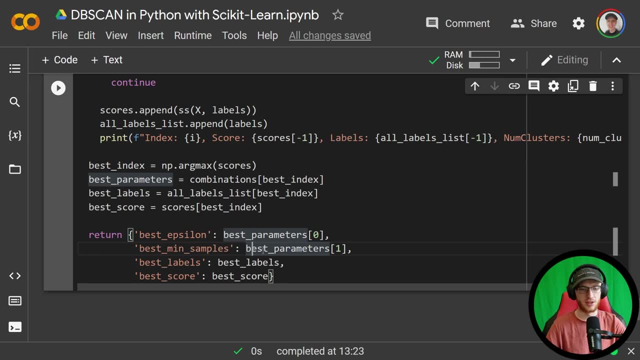 but it is done after. we simply just return this dictionary, which i'm going to do as return, we'll get the best epsilon, which is best parameters sub zero. it is going to be the best min samples, with best parameters sub one. since this thing is a tuple, we need to get sub zero and sub one. 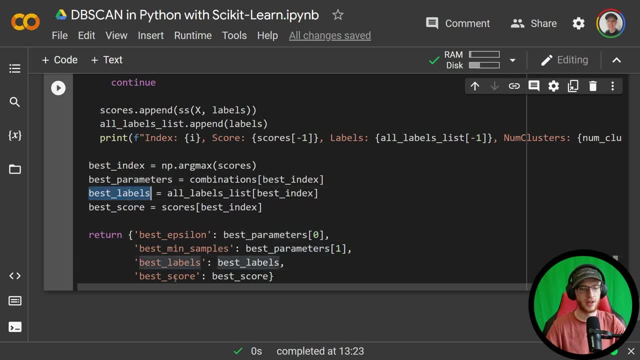 best labels, which is that labels there, and best score, which is those scores there. so we're just returning a dictionary, our results, basically now what we can do with this absolutely massive function that probably no one else is really using is best dict is equal to get scores, and 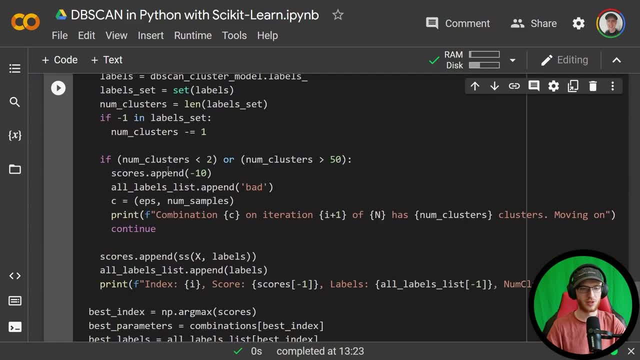 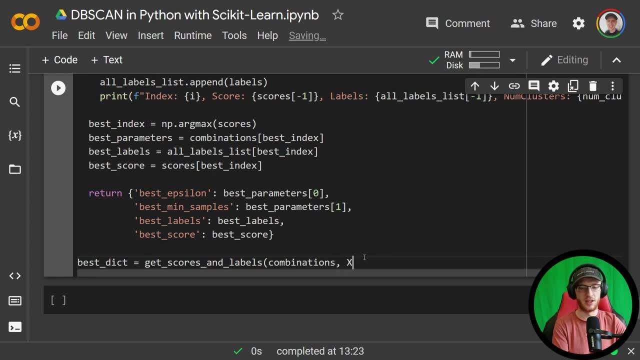 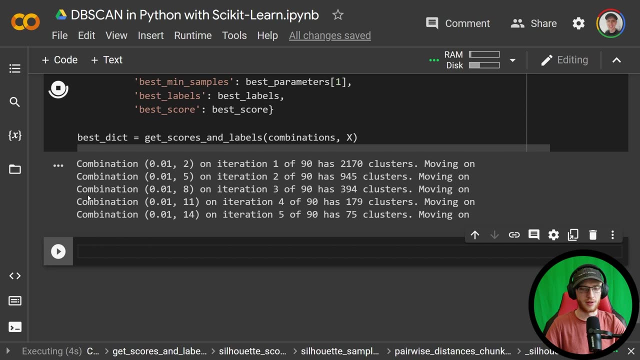 labels. that's what we call this function up here. get scores and labels. technically it gets a little bit more than that, but get scores and labels on combinations and x. now, if we run this, you will see that it takes a pretty long time and i probably will skip to the end, but it shouldn't take too long. 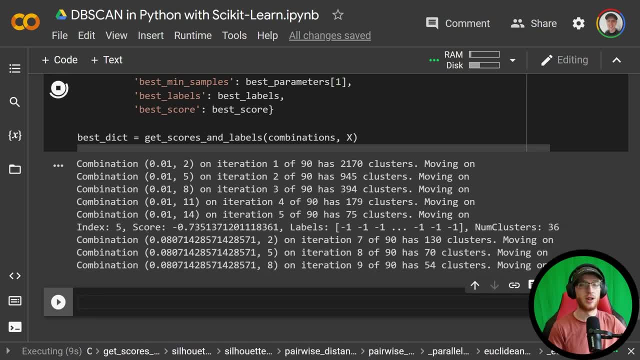 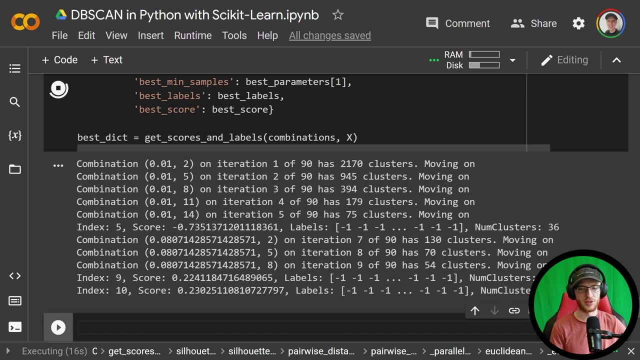 and i made sure that this doesn't take a massive amount of time. on google colab it takes a little bit to do a grid search. that's understandable. with machine learning sometimes you do have to wait a little bit of time, but with our output you can see some stuff being shown when i write moving. 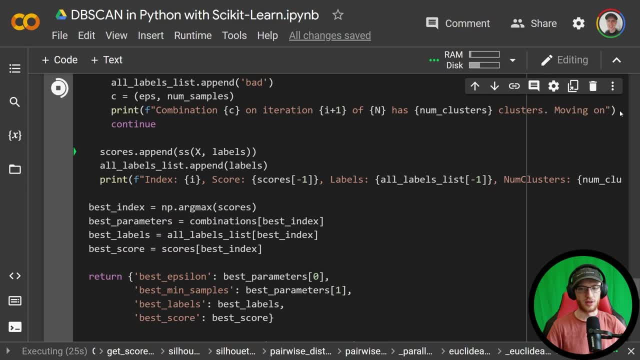 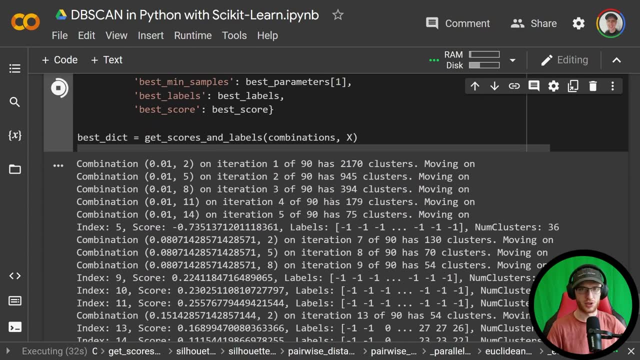 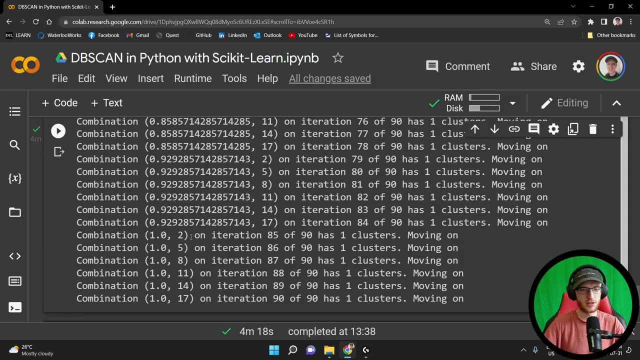 on here, that's our output. or that's: uh, that's our our printout here that says, hey, it has this many clusters. this is why we're moving on and we're not really, we're just adding trash and we're not actually, uh, thinking about that one. i will just resume the video after that's over, so as you can. 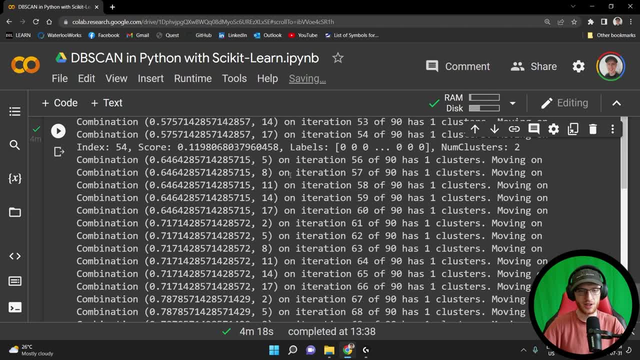 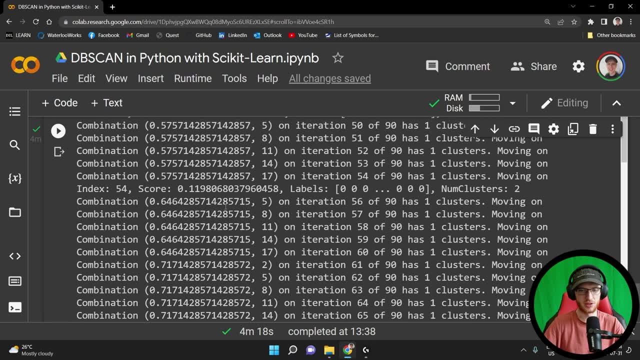 probably see if you followed along, even if you didn't. here you can see after it hits a point. basically, after the epsilon and pretty much after the epsilon, it gets too high past 0.64, so it uh, just getting way too high and it's just getting way too high and it's just getting way too high. 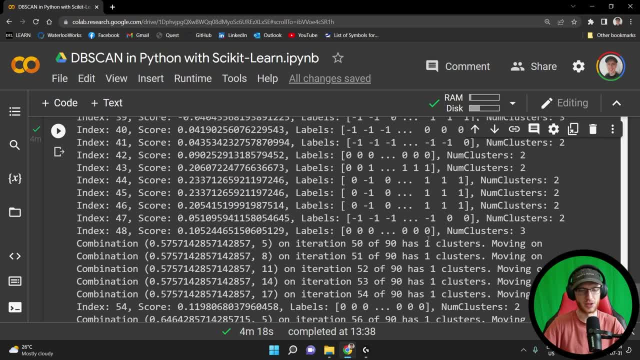 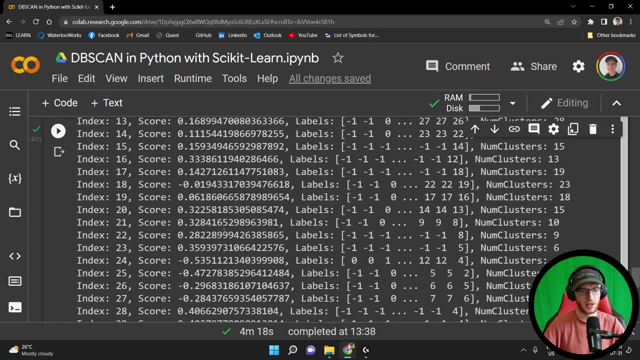 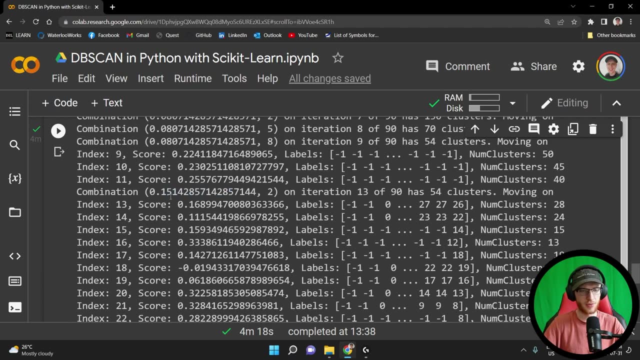 way too many or way too few clusters. it's getting one pretty much every time and so it pretty much gives up. but there is a lot of different, a lot of different options in here, especially in around this range where we have the epsilon. uh, where is it around around, this combination here around? 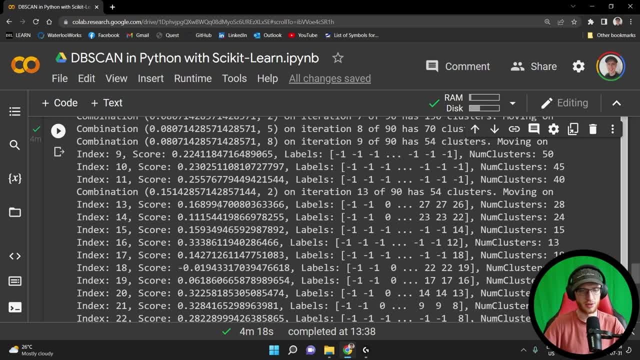 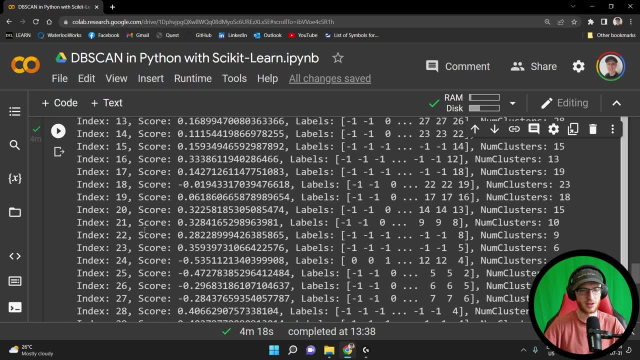 epsilon is 0.15 or so. with min samples different values. we're getting some pretty decent scores in here. we have a 0.32 uh and a bunch of negatives as well. it definitely varies, but you can see we are beating our previous score of uh. i think it was 0.25 when we tried it on our own. we're getting many. 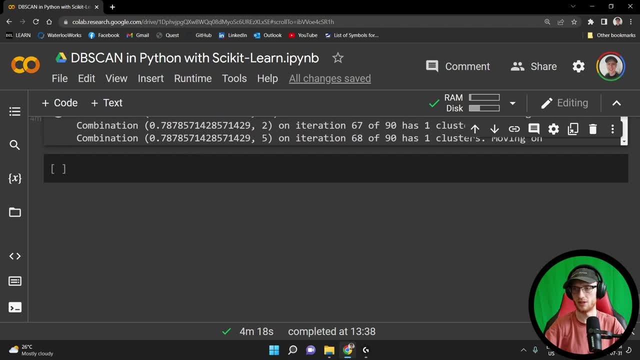 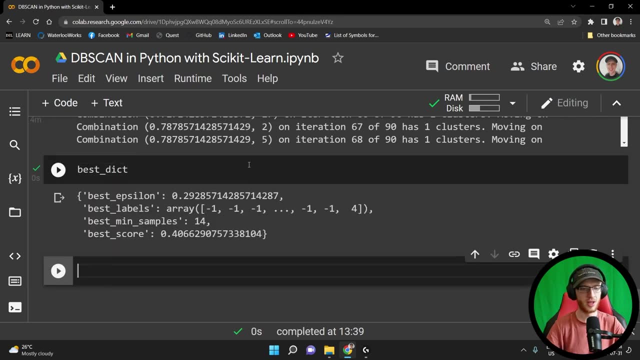 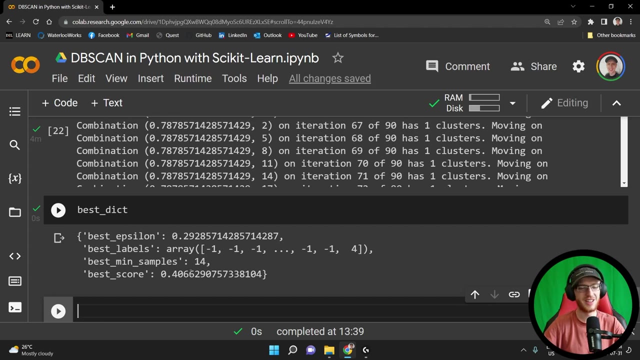 different scores that are higher than that, which is a good sign. that's, uh, that's the best we can really hope for. okay, so let's extract our best dictionary, because we got that stored in a variable. best dict is the best, epsilon is 0.29 and that is not true. sorry, that is true best i was. 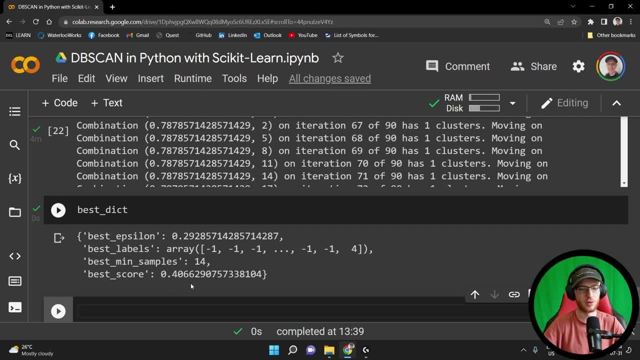 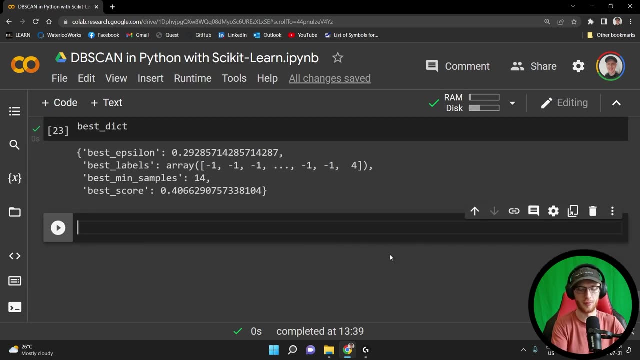 thinking that was the score. uh, best score, we found a 0.4066, which is much better. uh, these are our variables associated. we'll grab those and these are our parameters. epsilon is 0.29 and best min samples was 14 associated. now let's just go ahead and override what we had before, so we'll do df sub. 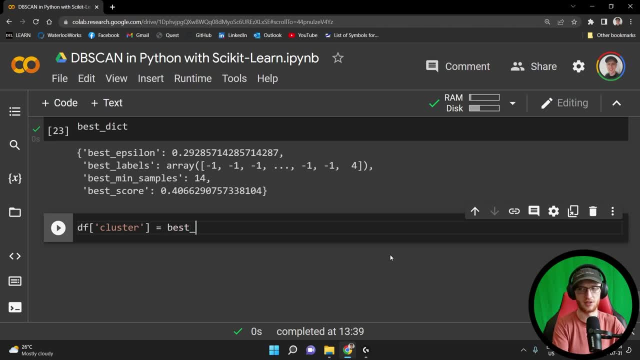 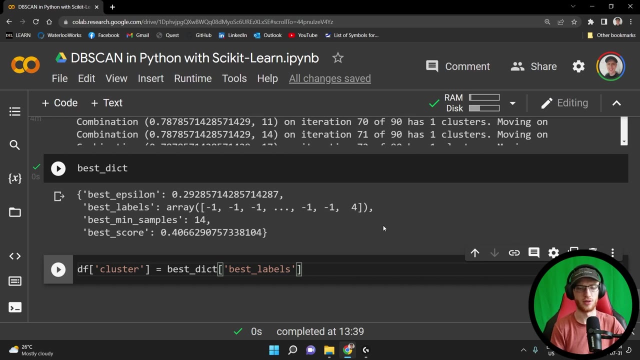 cluster is equal to now, the best dict sub, the best labels. really, all that we actually need is the labels, although we did store this other step because it's kind of interesting for you and i to see what values were actually making this work. maybe, if you wanted to further. 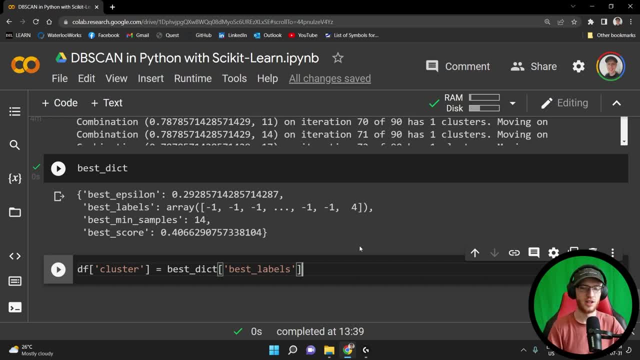 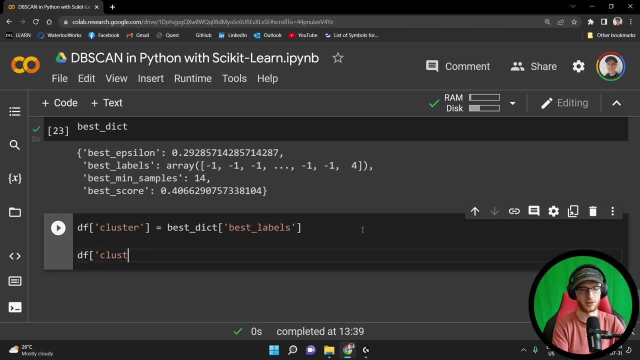 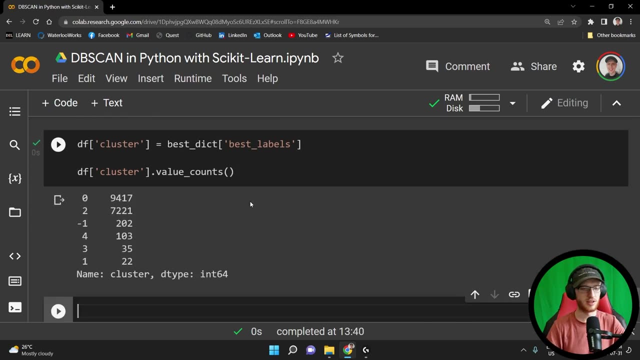 kind of do a closer grid search around these areas. you could do that. but really we're just going to take these labels and we will again look at the df sub cluster dot value counts, looking at the distribution that it was outputted and it outputted this. that's a nice amount of clusters. 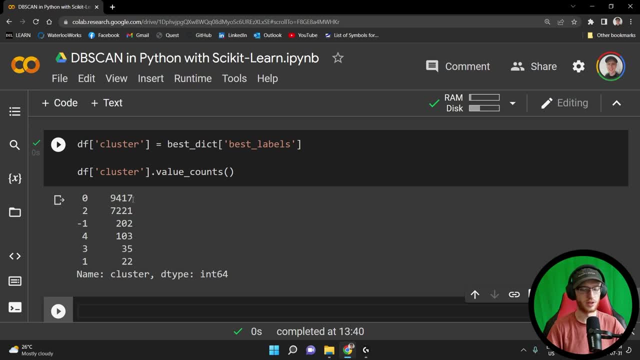 usually something like in the five or six range, is quite often a nice number and minimal noise, a little bit of noise 202. but if you do have outliers like that's, they should be clarified, classified as outliers and a nice different distribution. so what's good about this is there's not some or 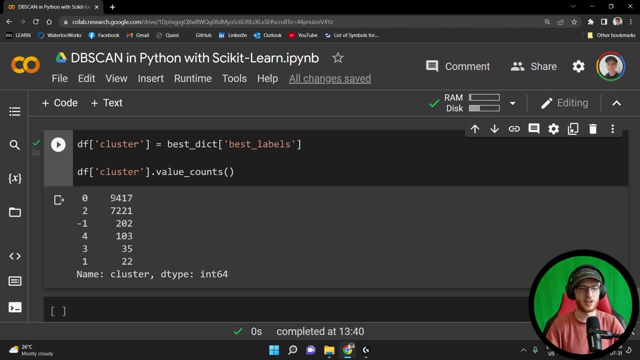 there's like so few, like we're not getting like three or four points and it's not like all dominated by just one cluster. we are getting mostly dominated by two clusters and then some various other things. so, just like before we are going to make our graph, and it's the exact same. 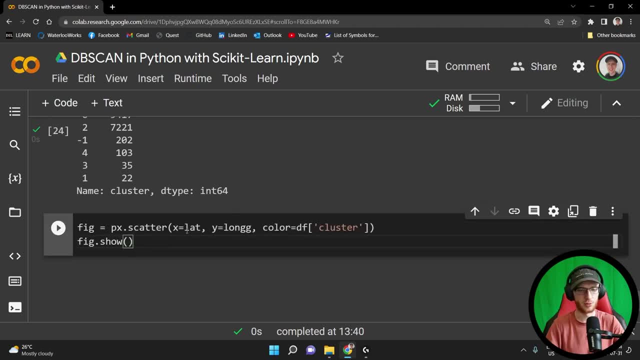 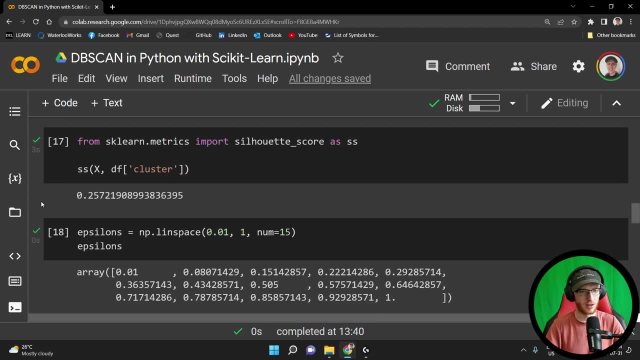 so i'll just copy it in fig is equal to px, dot scatter x with. actually that should be long and lat, i think, because i believe my code is actually wrong over there. we should be outputting it as: yeah, long and then lat, not lat and then long. sorry. 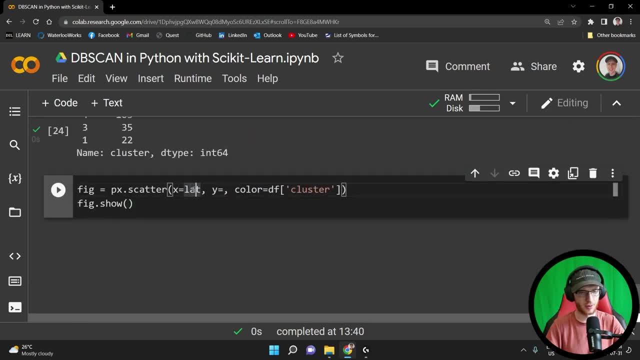 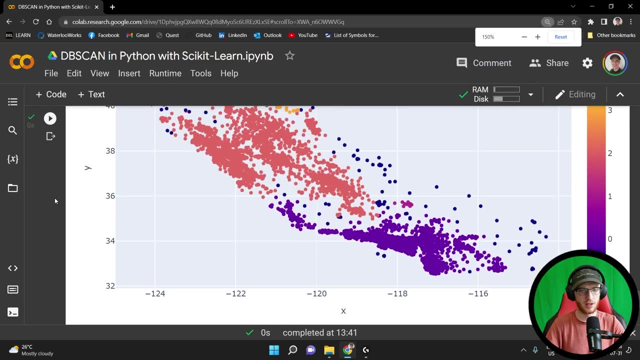 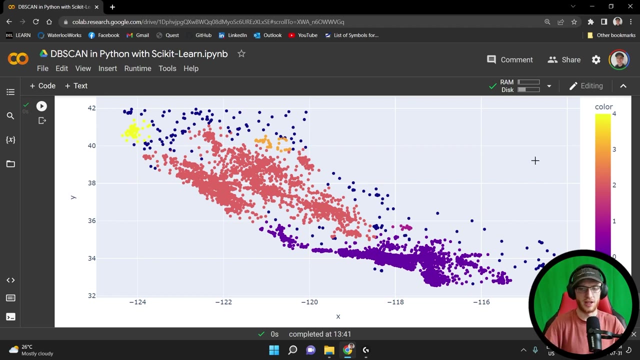 about that so long should be over here and lat over here, and then we output this again and we see something that maybe makes a little bit more sense. you know, i think this color it's definitely better than um one of the earlier ones we've seen and that first one, you know, i think the first one. 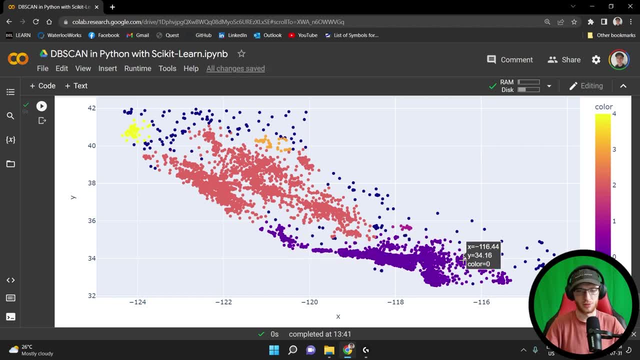 didn't really make too much sense here. you could kind of see some, some uh distribution over here. another cluster sort of makes sense in the middle it seems to have. i'm kind of surprised it found one over here and that wasn't classified as just pink, uh yellow. i can definitely see why. 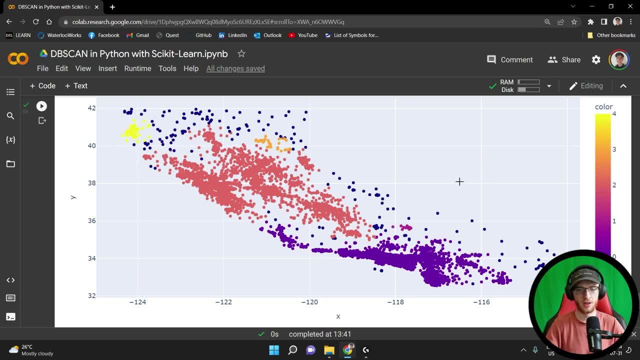 they're just kind of its own cluster in the middle over there and everything over here is classified as an outlier, which is really what we wanted to see, because the stuff on the outskirts that kind of did strike me as either maybe it could could be marked as its own cluster, or if it's not, then 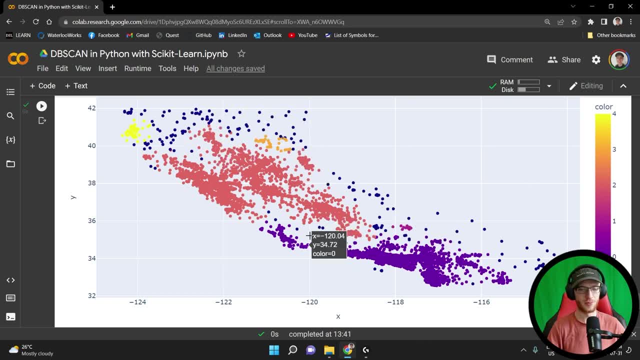 at least it should, all around the edge, be kind of classified as noise instead of some of the other stuff in the middle here definitely just seems like that one. you wouldn't really associate that with anything other than an outlier. okay, so this is just kind of showing you that you can actually optimize to make a, um, a visual cluster model that actually 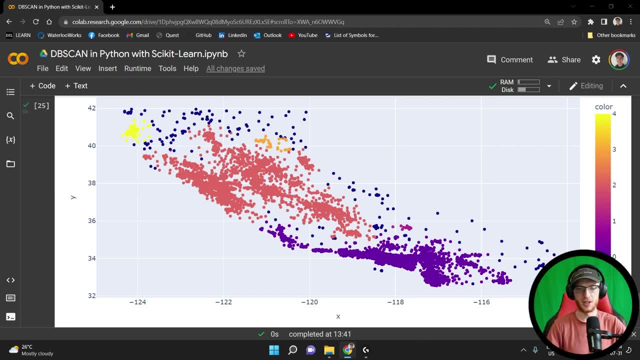 makes sense. now, a big question here is: well, what if you have more than two variables? because you can't really, you can't really color this and you can't really visually look at it. well, if it's more than two variables, well, you would actually just do the exact same thing that we had. 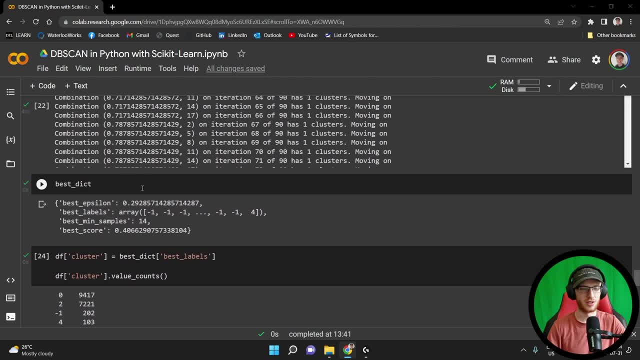 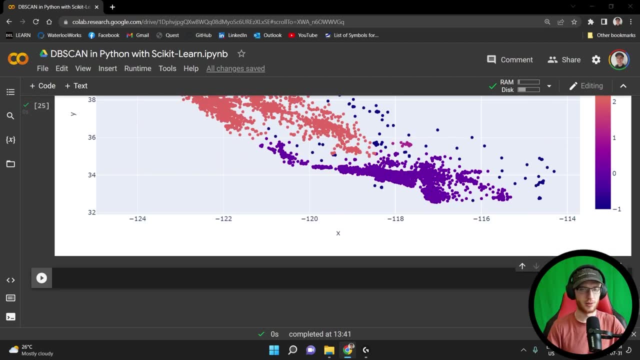 before. you wouldn't really need to change anything at all because we optimize this for the silhouette score. however, one thing that you should change, even in our example, it wouldn't probably wouldn't do anything, although it doesn't hurt because it's a latitude and longitude. i said it earlier. you 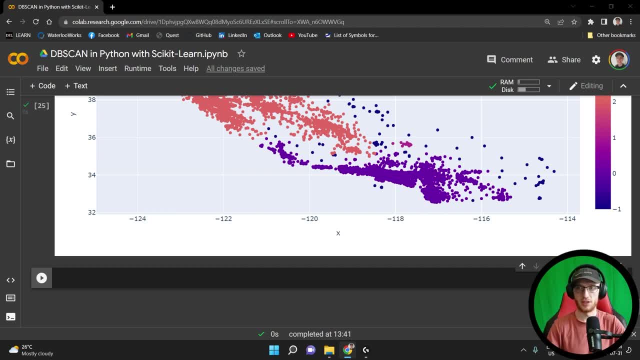 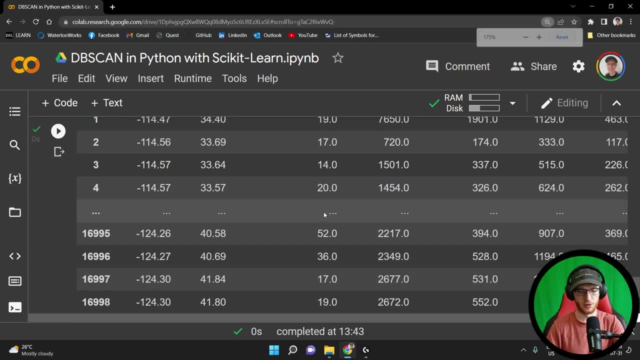 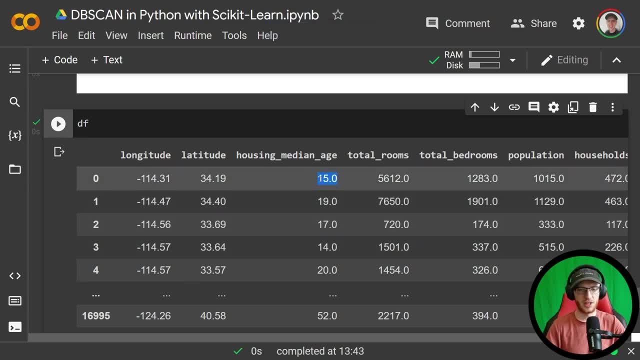 at df and you did try to do a clustering on this. well, housing median age- age is generally very small. you're not going to get a housing median age bigger than like a thousand or probably not even close to that range. but if you have total rooms and total bedrooms you'll definitely be. 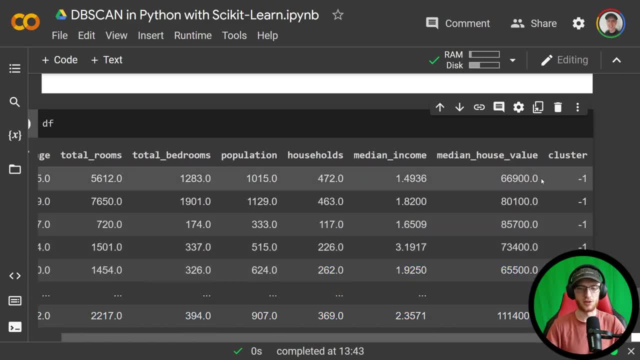 in the thousands and other variables here, especially if there's money involved. money is very, usually a very large number, and so median house value, if you had that in there. you have some variables that are on a very small range, like zero to a hundred, and you have other variables that are like zero to like a hundred thousand, and so basically, basically what? 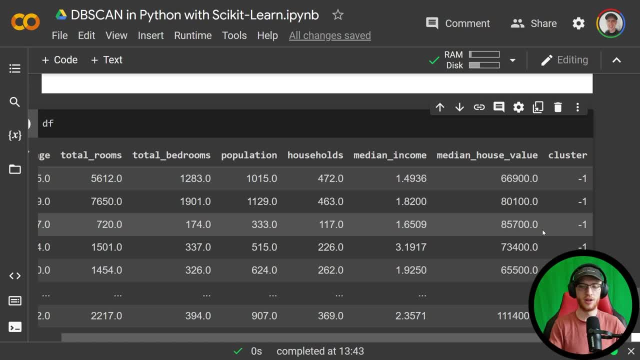 would happen if you just put that raw into the algorithm. well, it's just going to really ignore those smaller, uh, those smaller pieces, because the distance between, say, this point and this point is like fifteen thousand, but the distance between, um, like this variable, this very, this variable is. 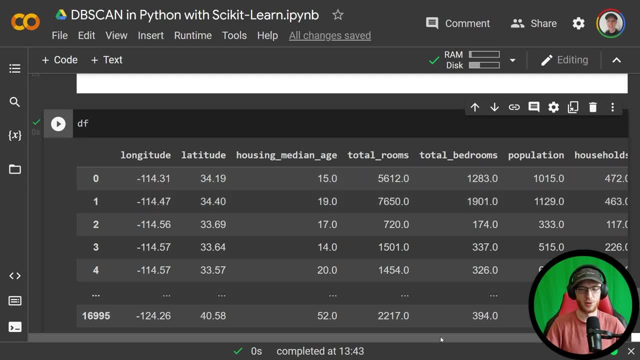 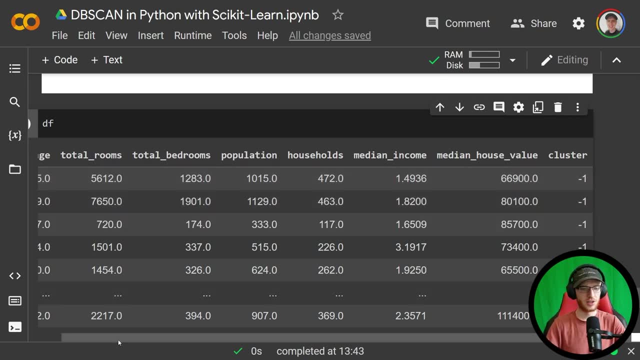 only four. and so it's going to say like, hey, i really don't care about this four distance, when i have to maximize this, when i have to worry about this fifteen thousand distance over here. okay, and just to show this graphically, i will pick a couple of variables. that explains it. 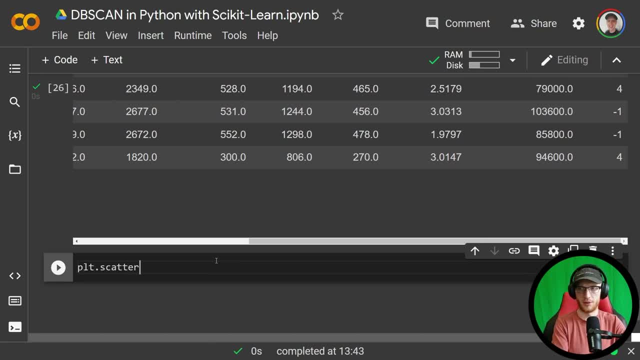 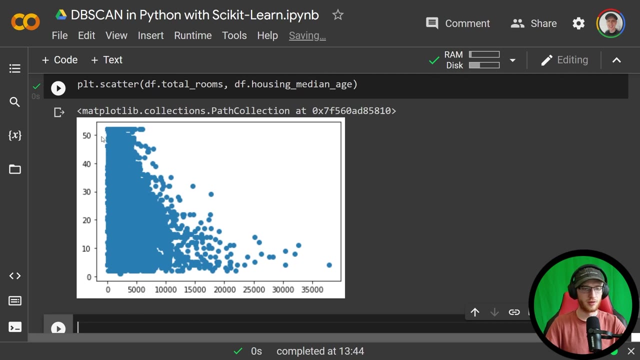 very well, you'll do a plt dot scatter on df dot total rooms- that's one column- and df dot housing median actually. yeah, i'll just stick with that for now. it's good enough. okay, so here you can see it's kind of all slanted over here, but most importantly you look at the range of the. 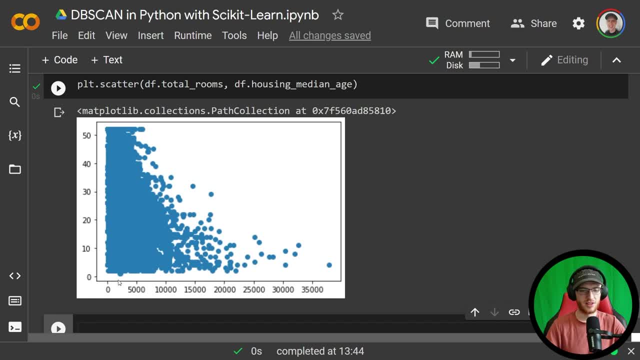 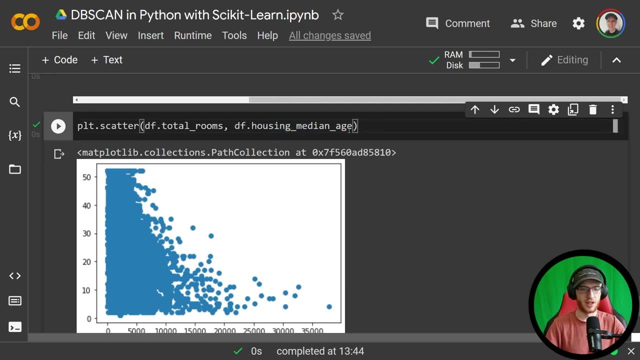 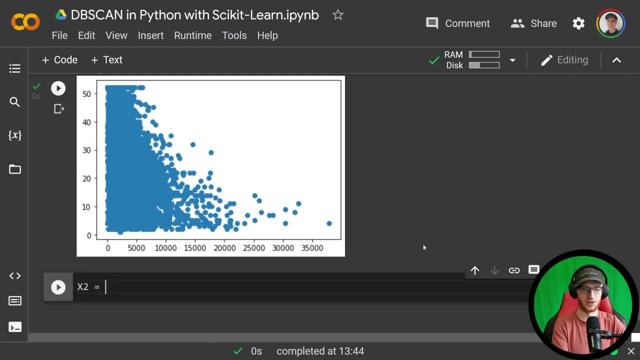 x's, as we just explained, zero to sixty or so and zero to thirty five thousand or so. the db scan algorithm would be completely dominated and generally just confused by these different columns here. and i can show that if we were to do x2, so just getting another matrix here, x2 is df. 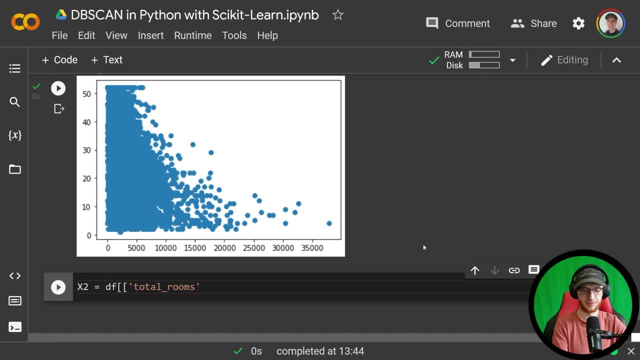 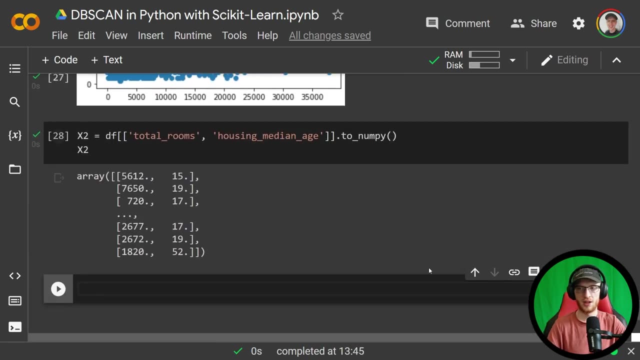 with those two columns- total rooms and the housing median age- and we put that, converted that to numpy and we'll just show x2. now that we really need to show that that's x2- a different matrix- and we will, since we have that awesome function from before. that's why we put in so much work to get. 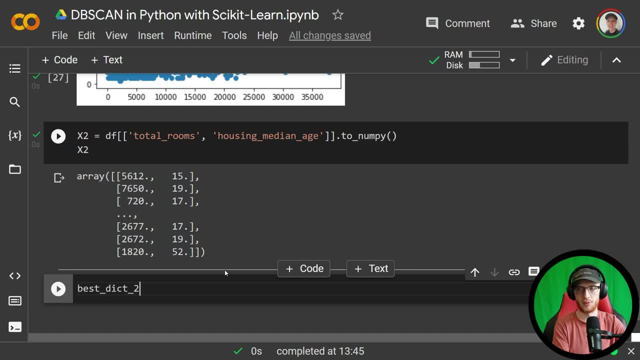 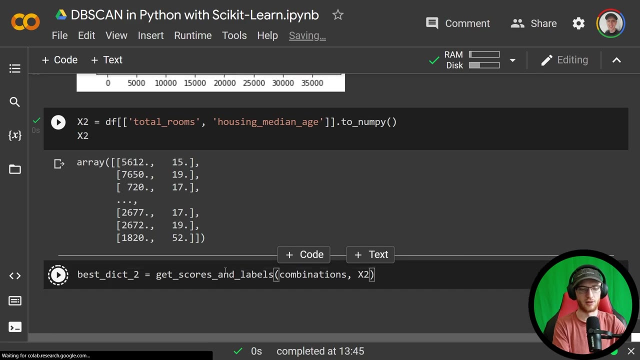 this great function we can just do best. dict two is equal to get scores and labels calling that function. if i can type it- get scores and labels with combinations and x2- then we should be able to do that, and then, while it's going in a new set- okay, it's not even letting me type, so basically: 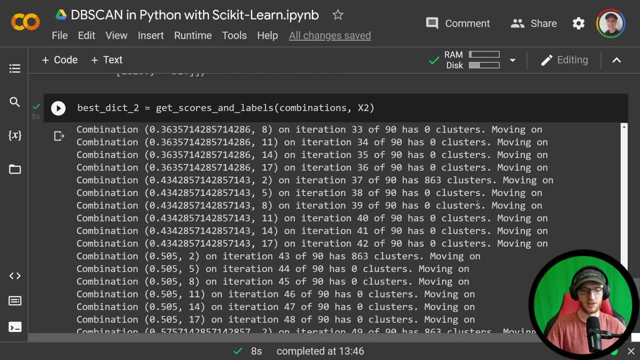 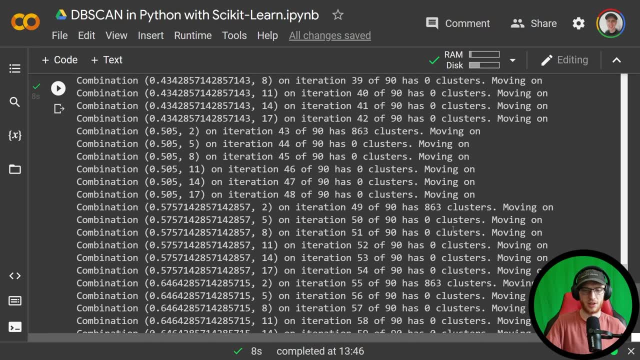 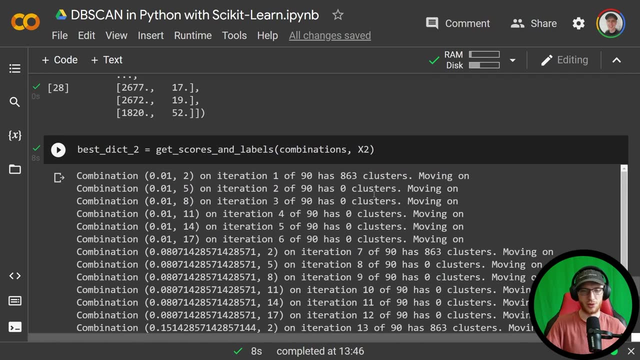 the point here it's moving on. every time it's: uh, it just finished because it didn't really do much of anything. it kept making these models, but it kept having zero. here's zero clusters we're getting, or this is 863 clusters, and so it's very, very confused here. you see, most of the time we're 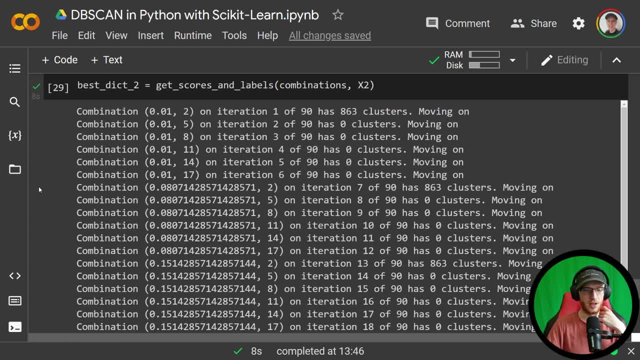 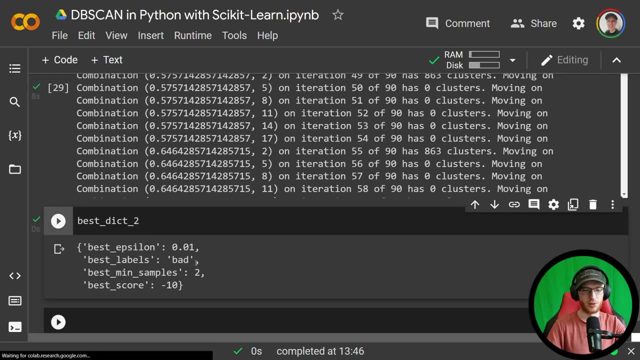 not getting any clusters and that's because our scaling is really messed up here, and so if you look at which i tried to do best, dict two, uh, we're, we're stuck with bad. okay, we have in best epsilon and a best min samples, which is the first one because that's associated with garbage and that's. 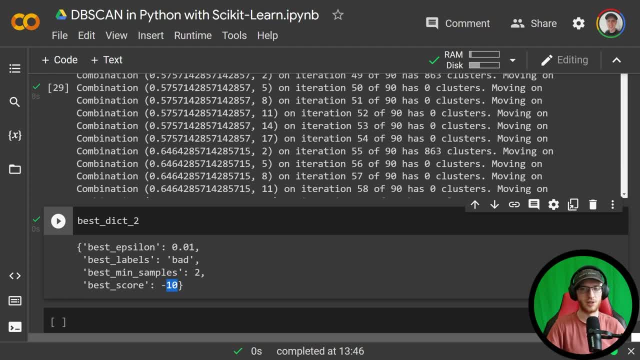 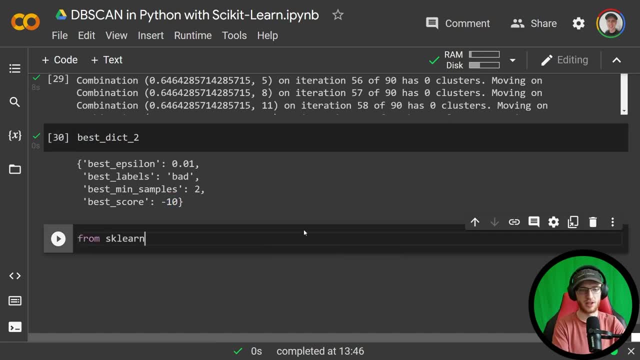 because literally all of it was garbage. there was not a single cluster model that really made any sense, and so if we do go ahead and scale our variables instead from sklearnpreprocessing import standard scaler x2 scaled is equal to standard scaler dot fit transform, we don't really need to keep the 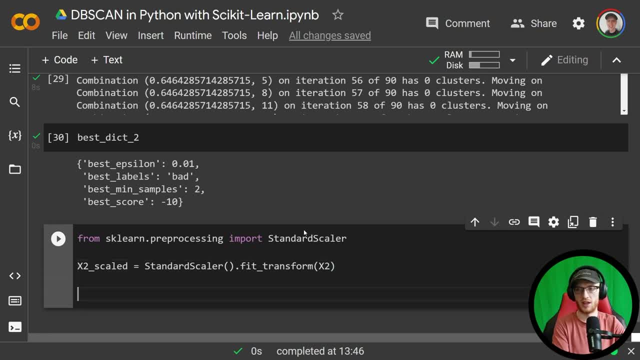 transform. so i'm just going to do a fit transform like that and not worry about it. after plt dot scatter x2 scaled will show all of the first column there and then all of the second column. just a different way of showing. we're just scaling the variables and then we're using. 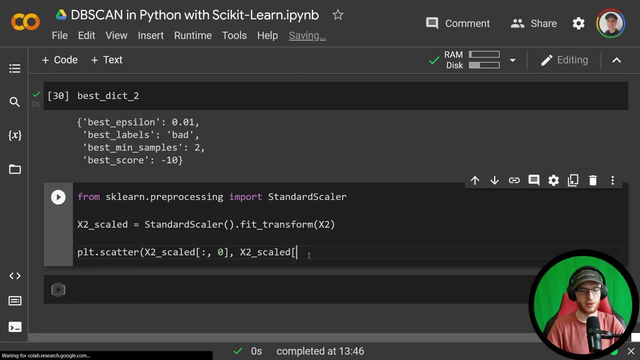 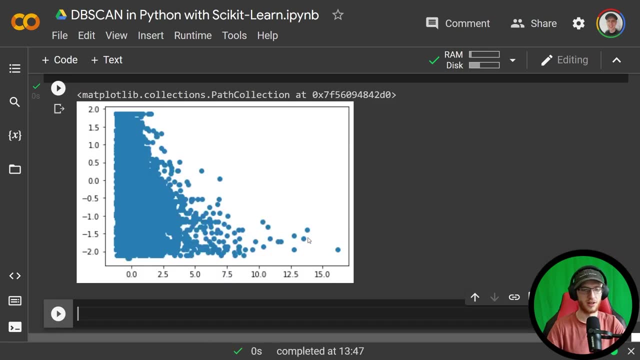 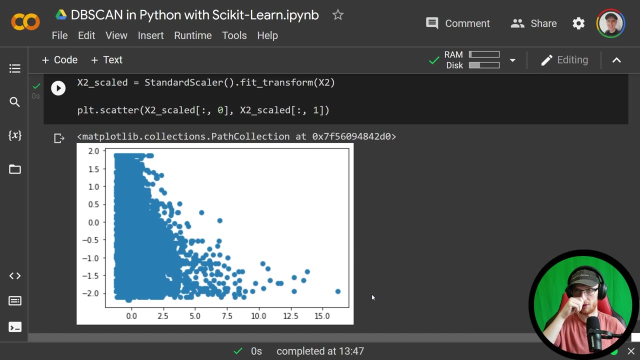 the standard scaler in particular, and we are going to graph those. so this is the first column. second column, all the rows and the second column, plt dot scatter that it looks the same here. it's still going to have that shape, but if you look at the range here it's much, much closer. still not perfect but, uh, much closer. 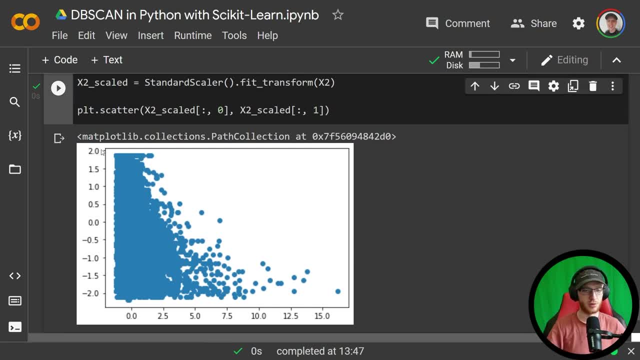 and so this is zero to negative two, between two and negative two, or maybe negative three and three, and that's, this is about negative one to about 16. so again, not perfect, but they are much, much, much closer to each other. and that basically says to the algorithm: hey, we're going to treat these uh. 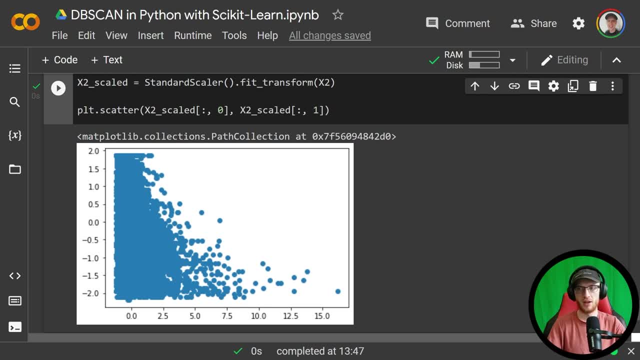 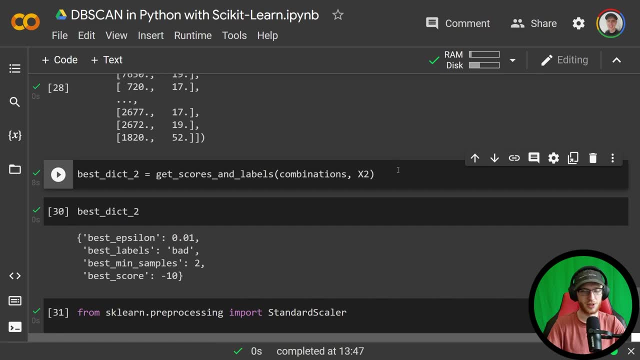 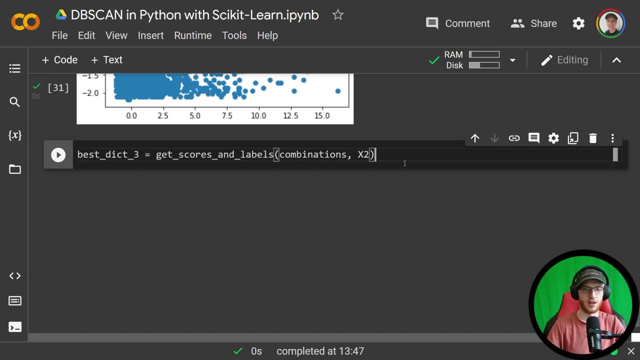 relatively the same as the same as we can. we can get uh, and now what we can do is just that same thing as above. so i'm going to copy this exactly. i will remove that. that's way too much. writing best dick two: i, i could make it. we'll just make it best dick three. that's, that's a three, uh, and 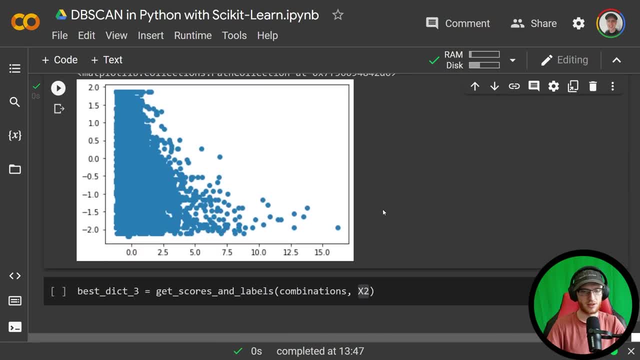 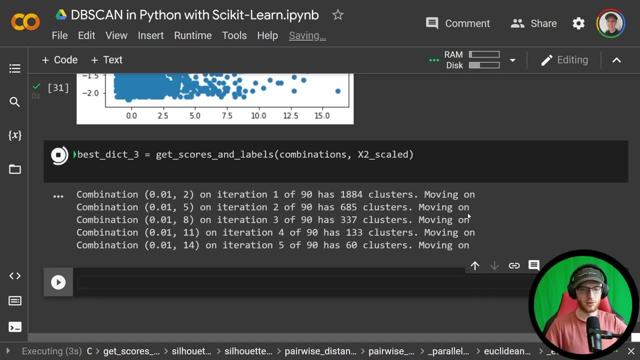 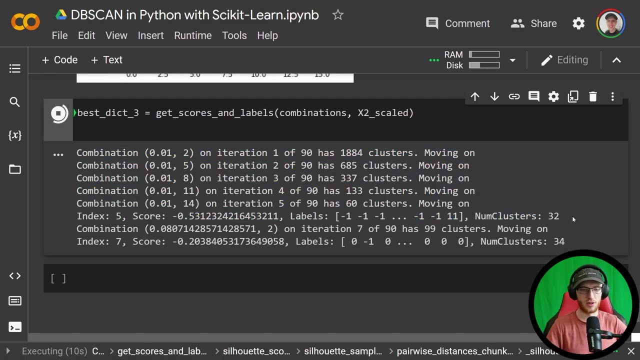 then this should be the only change that we have to do is x2 scaled and let's let that run. now what we're going to see is, sometimes it still runs into trouble. we don't expect these clustering algorithms to be magical, but hey, index five, here we did get num clusters with 32. 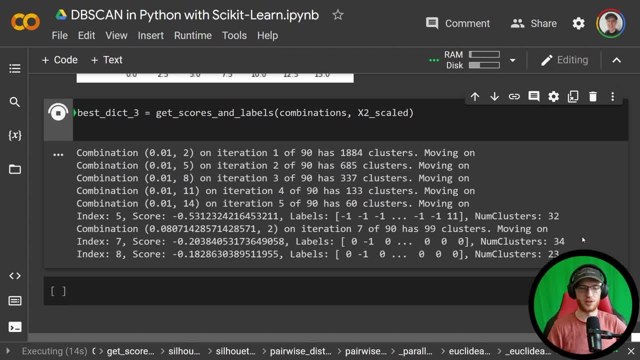 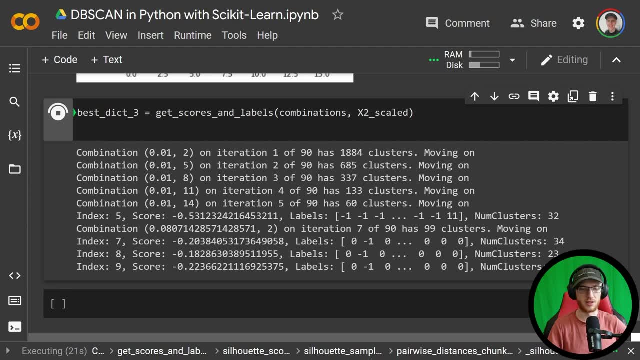 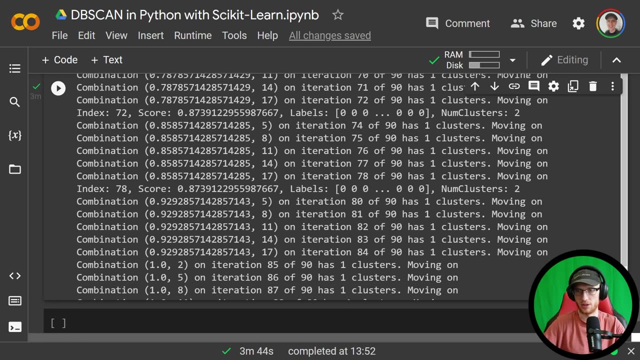 54 and- sorry, 34, and so these are looking not so bad and i, since it's actually working again, i will jump to the end of end of it, since this is going to take a little bit. okay, so we're all done over there, and what's nice is there's many different uh scores that actually were not too bad uh, and 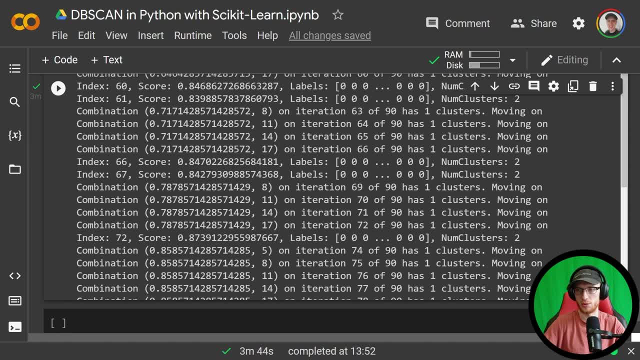 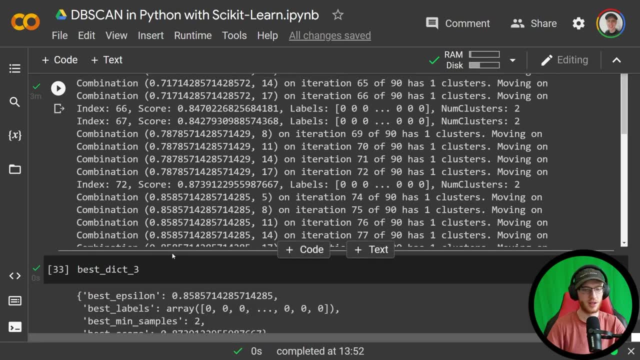 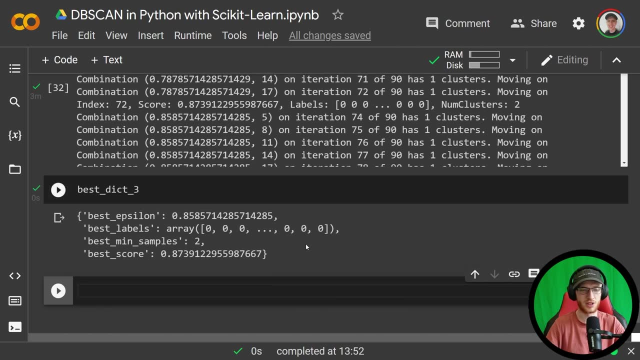 i'm not really. i'm not really concerned about the actual score, although we will take a look at it. we can take a look at best dict, what is now best dict three, and we see these different options and what we can go ahead and do is- i'm not going to overwrite any of the columns because we're 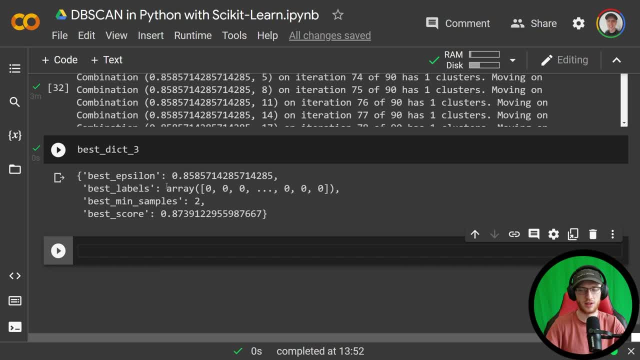 just about done here, but we can take a look at the uh, the new coloring, and so we will just make a new fig equal to the px dot scatter with x is equal to x2. underscore scaled uh from zero. sorry, all the rows, and then the first column, y, is equal to x2. 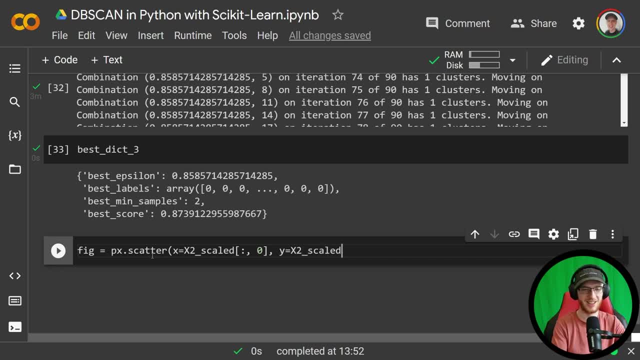 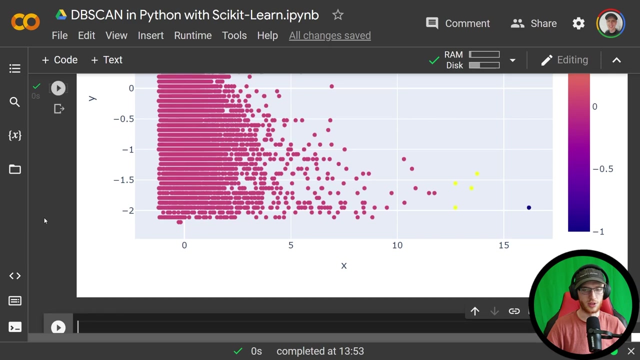 scaled like what, sorry, um colon, first column and color is equal to best dict three, uh sub the best labels. okay, we have those labels score stored in there that we got from our optimization and we should just be able to do a fig dot show, which might not make perfect results, but it should make something okay. so this actually: 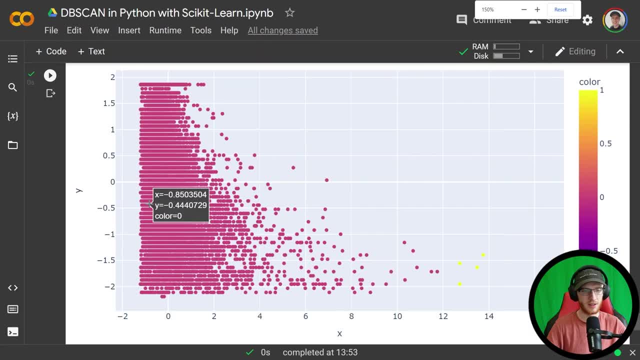 kind of makes sense. we have all of this stuff over here got assigned to the zero cluster. all this stuff over here, just these four points, got assigned to that one cluster, and then we have some outlier over there, which is really nothing. so it not to say that you can make some clustering. 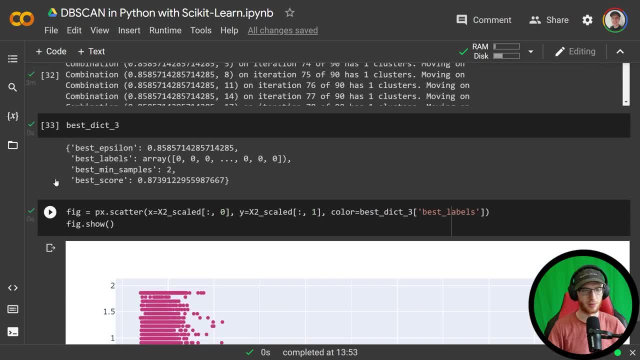 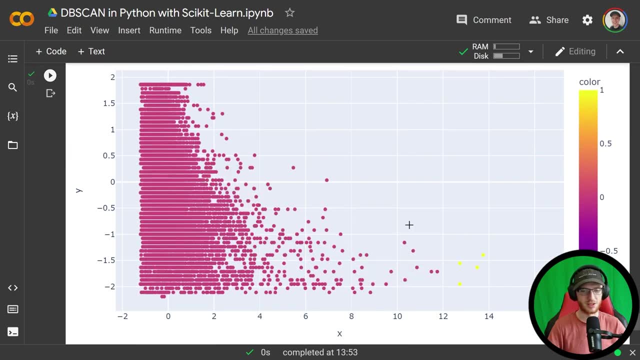 that really, really makes sense for anything. and you can judge that by the fact that, yes, this score. well, actually it thinks that the score is very good, uh, because you know you can see it does kind of picture good. whether that means anything it's kind of hard to tell. that's up to you, um that. 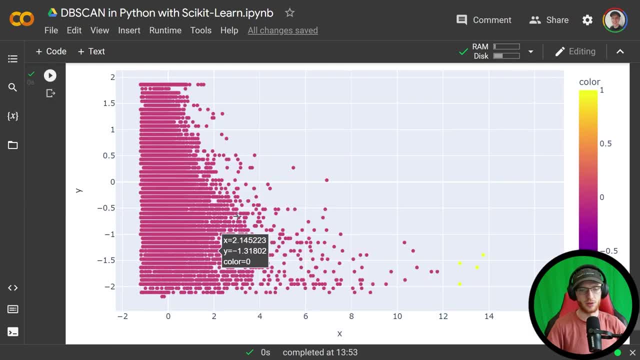 is. that is a good silhouette score. since we did scale the variables, we at least got something, and so the lesson is that you should always scale your variables, um, unless you're purposely trying to make a mismatch and to try and treat one variable uh more than another most of the time, 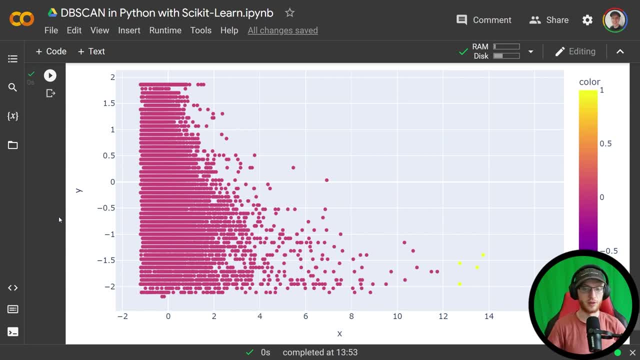 we're not trying to do that and you want to treat them as well, letting the algorithm figure out. uh, what's what's most important to really think about? okay, so that's the, that's the idea. um, i think it's pretty cool. db scan is uh much different. 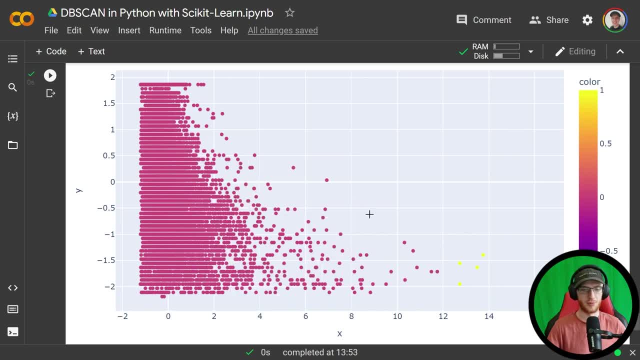 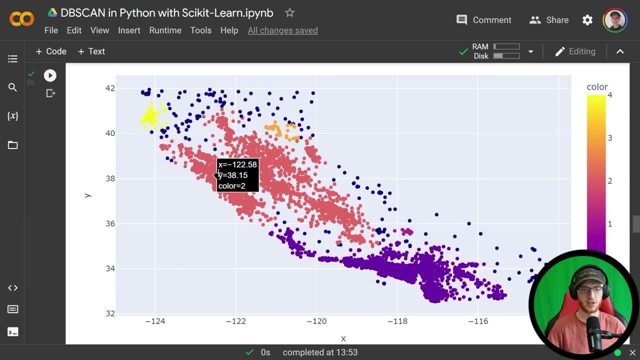 than k means because it's it is able to say all of these ones. actually it's mostly in uh, in going to be shown in this california piece. here k means uh. you would have specified the number of clusters or maybe done a, an elbow method, to figure out: um, what's the best number of? 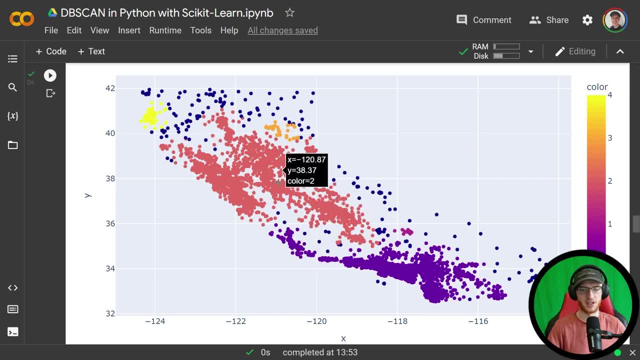 clusters, but either way, it would have kind of done: hey, this is an area, this is an area and this is an area, whereas db scan allows you to have these little pieces and flagged noise as some of the outside stuff. it's a very nice algorithm and i hope you learned a lot about how to use it. 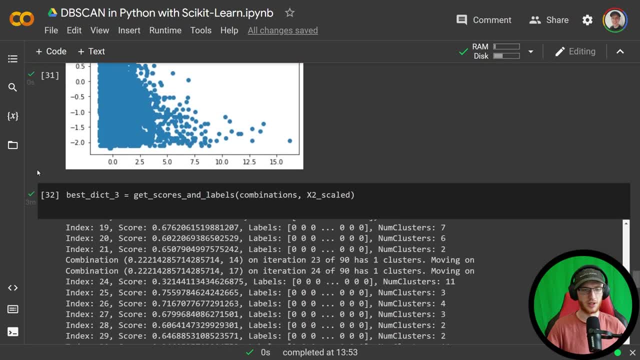 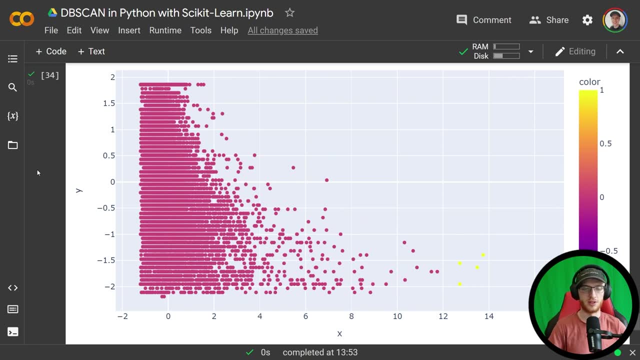 you can, uh, feel free to copy that function that i, that i, made, and scale your variables and use it, because it is. it will work very well and you can compare them via the silhouette score method on what is best. most people genuinely will not show a tutorial that actually shows you how to make a good model in db scan.